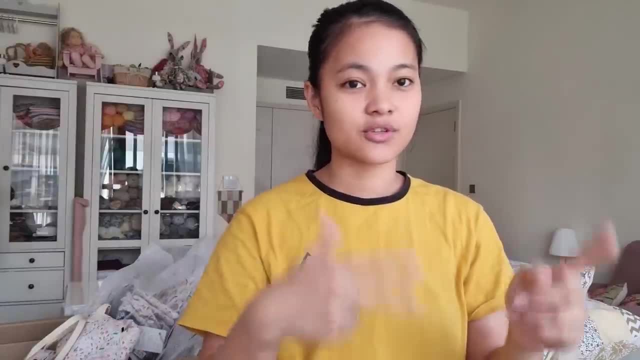 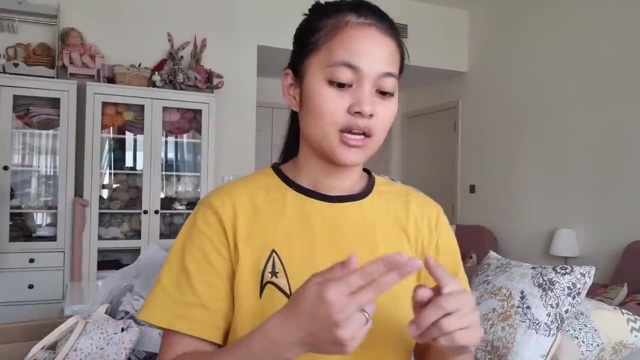 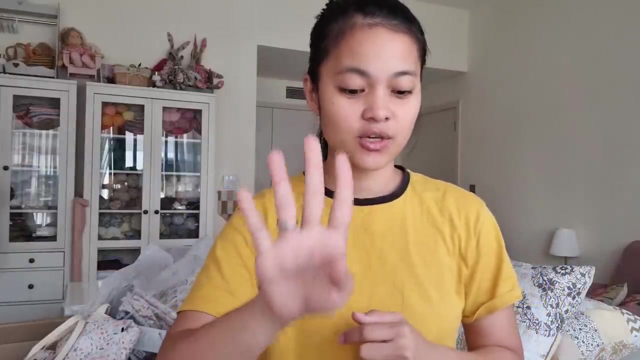 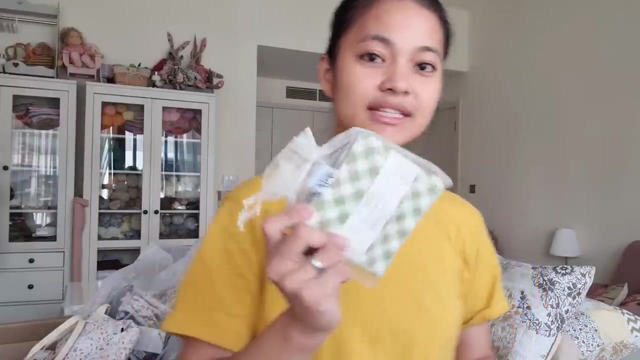 cheap to get the materials, you know, and also cheap- cheap when it comes to buying the materials. And fourth is it looks nice. So those are my four main things to you know that I consider when I'm selling Right. so just like this coaster, it's very easy, you know, it ticks all the criteria. 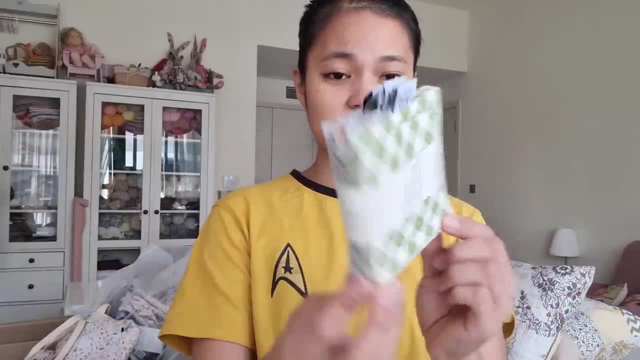 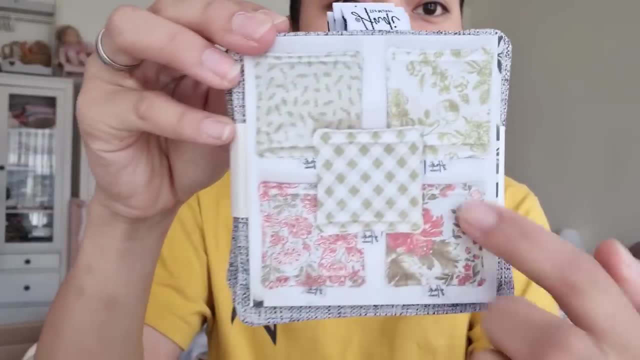 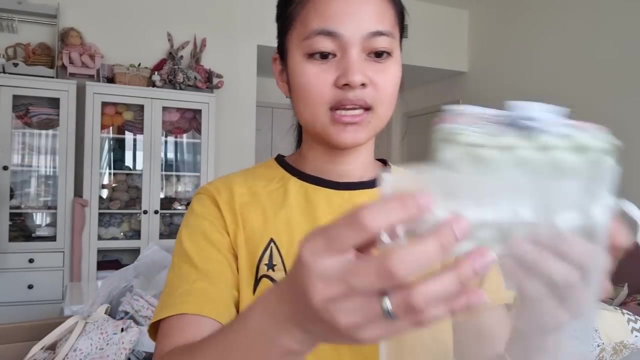 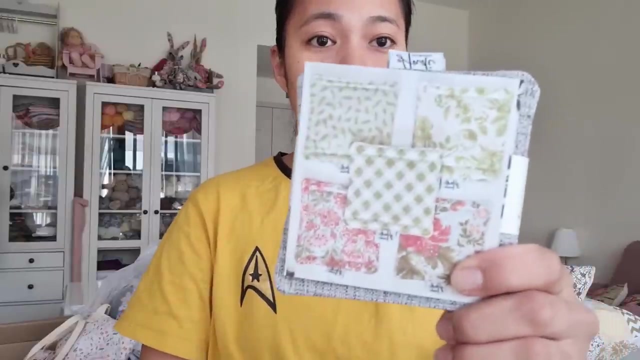 And it looks really pretty. So it comes in a packaging like this. Isn't that adorable? And at the back you can see all the colors That you will get in this pack. because it's already packaged- Well, it's in this mesh bag. You can't really touch and see what's inside, So I printed a photo. 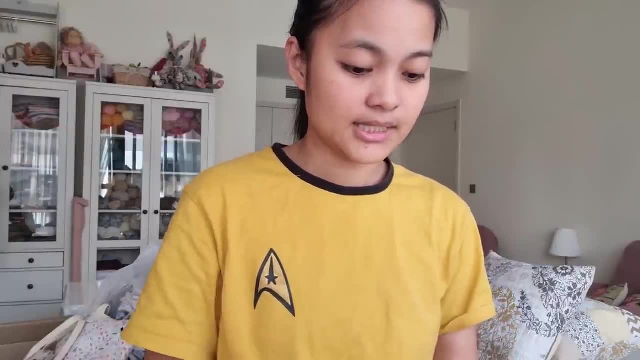 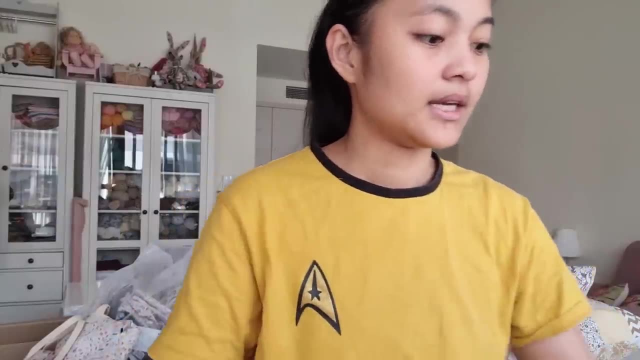 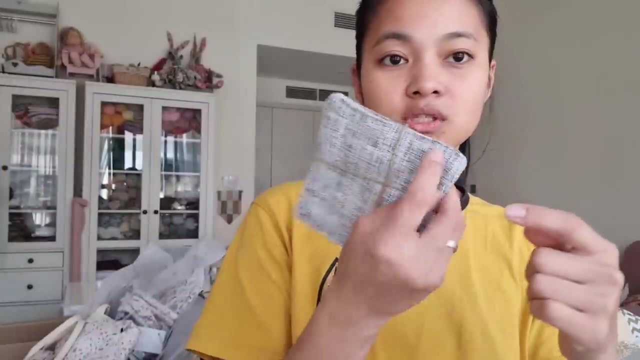 So I think that's brilliant, Right? So let's move on to the next one. They call me the pack of five, Right? This one coaster. This one is another coaster, But this. this time I've made the front and back from a curtain. 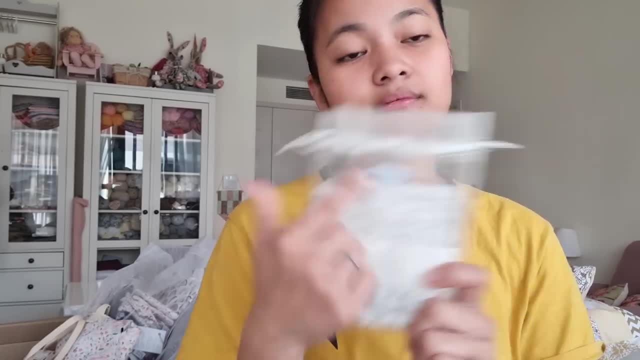 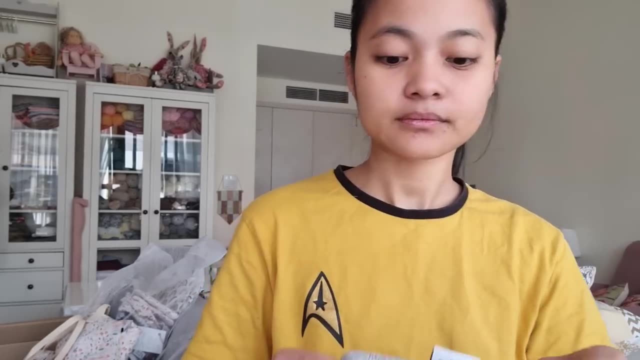 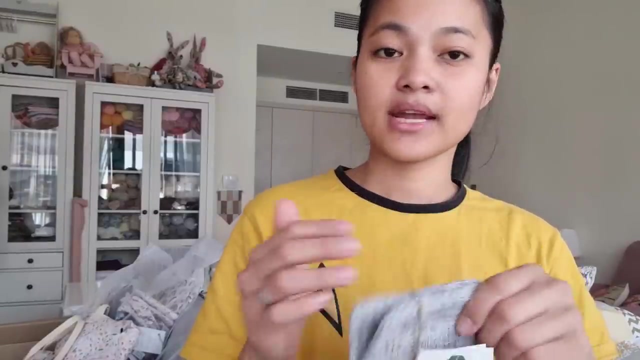 These printed ones. this front is sort of a new fabric and the back is from a curtain, Same fabric as this one. So these come in two pieces. It's great gift, It's just, you know, it's nice to have. 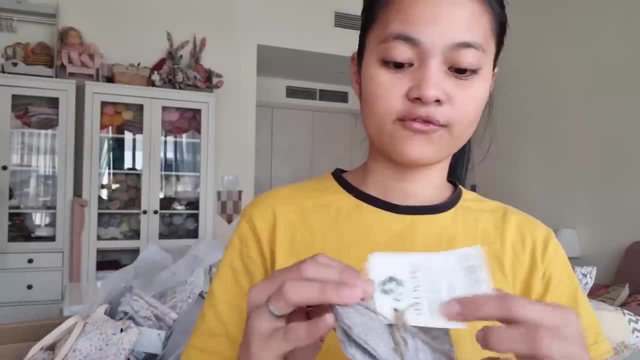 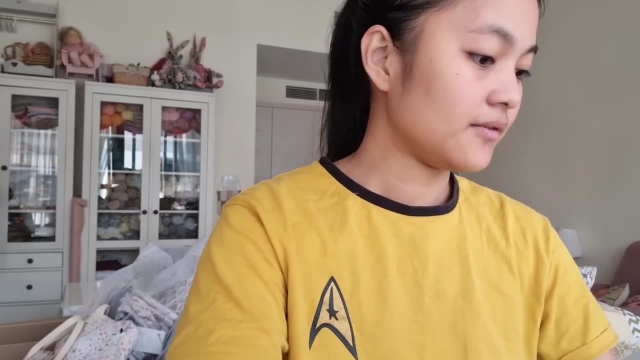 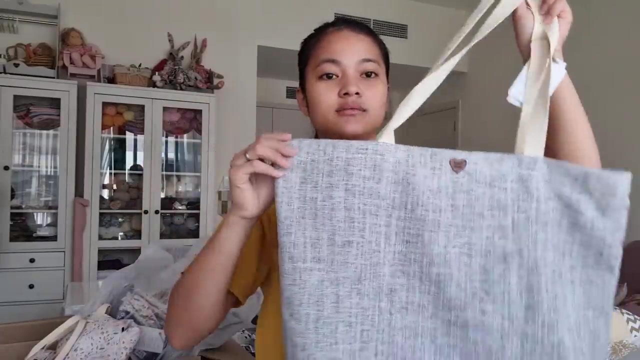 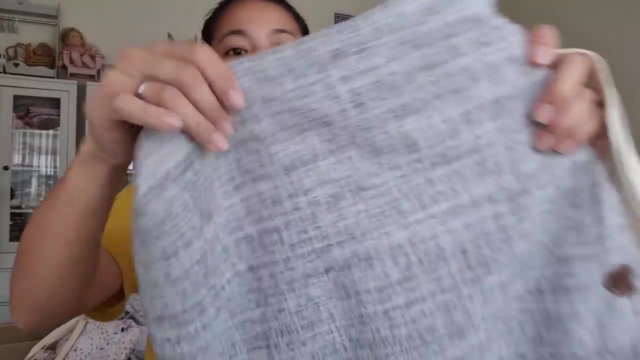 And, yeah, easy to make. I sell them for 15 dirhams for two pieces, That's. I think that's very reasonable And very, very easy to make. Now let's move on to the tote bag. Everybody likes a tote bag for market, for everyday, everyday. use it. This fabric is gorgeous. Look at that. 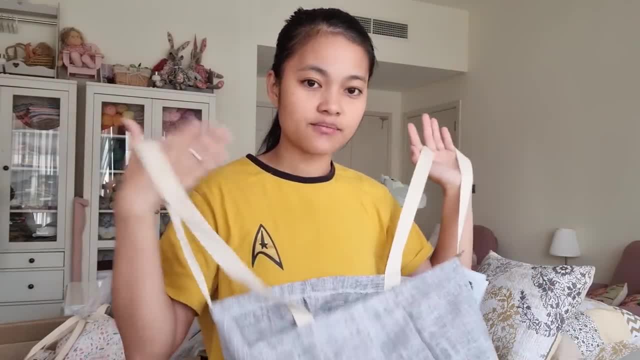 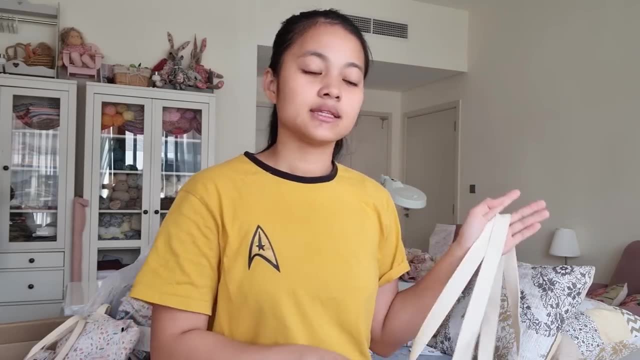 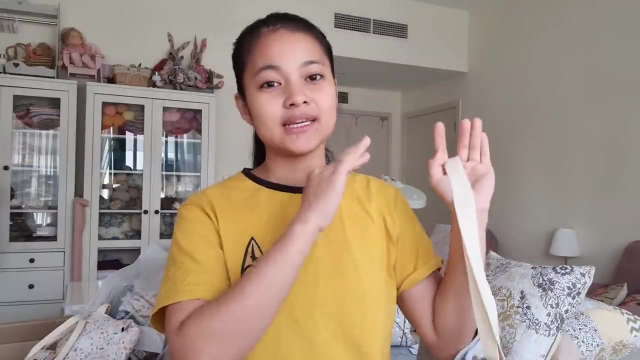 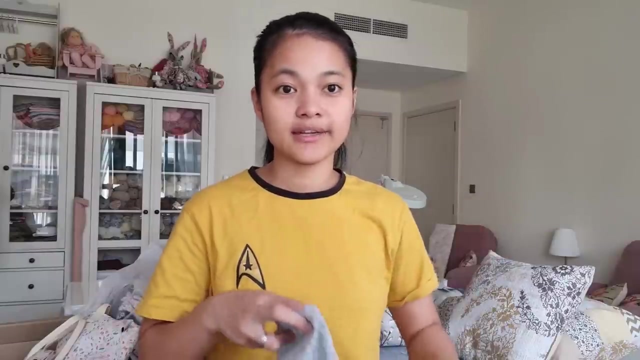 curtain. so some curtains i've bought um from, you know, from people living in dubai, and others have been donated to me and they are aware that it's for repurposing and upcycling. whoever you know those kind-hearted people are, they know that i'll be making and selling. 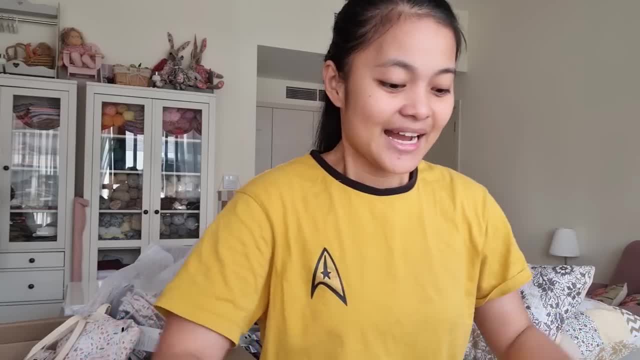 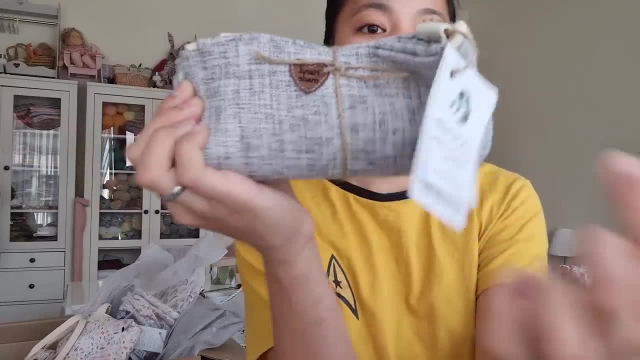 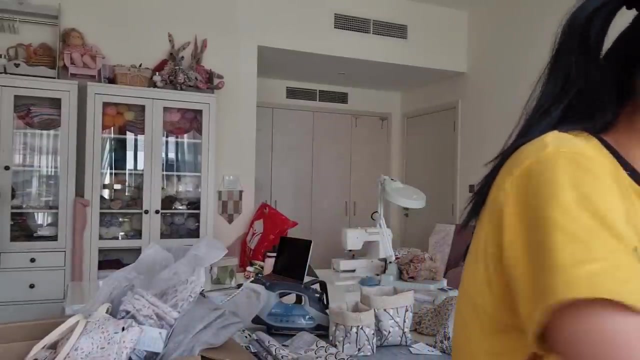 it's just nice to be transparent, all right, um, that's another one. so i've made them into a pack like this. it's got a little tag called it says upcycled. so yeah, right, what do we have here? so i made a few of these. i didn't make a lot of these because it requires a 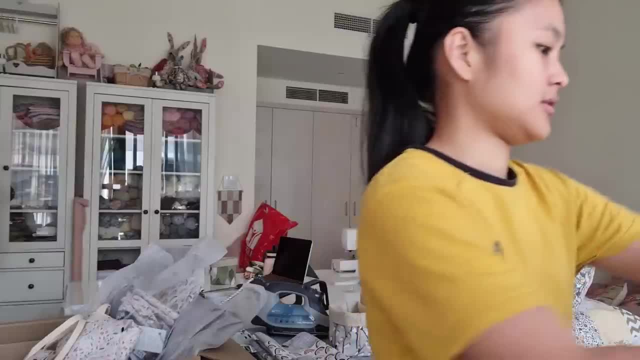 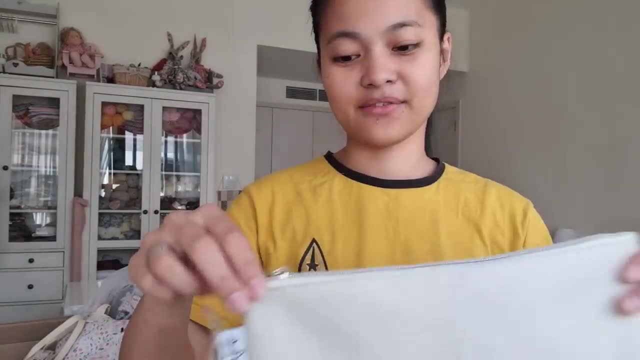 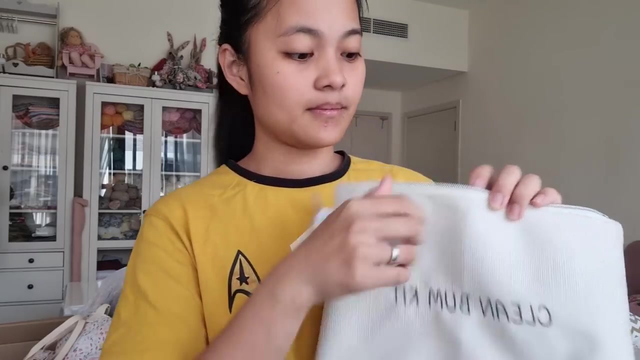 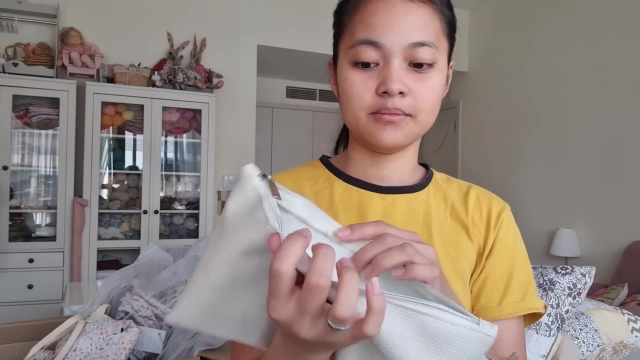 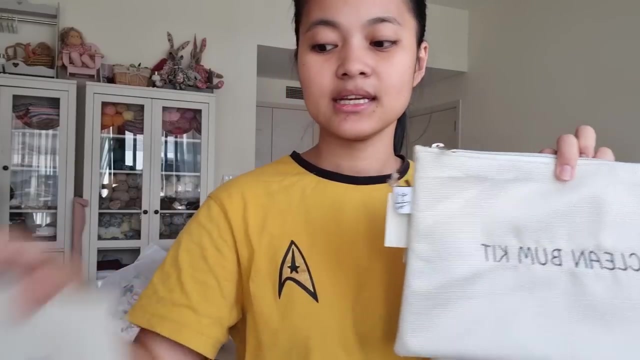 big fabric and i didn't have a lot of fabric, so i just had to make a few pieces of those. now this is my favorite clean bum kit pouch. so again, this is made from a curtain and it's not lined, but it's got this waterproof fabric, which is nice, i think. so that i made two of those and 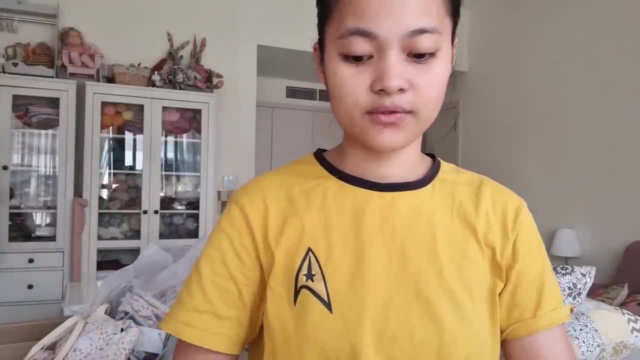 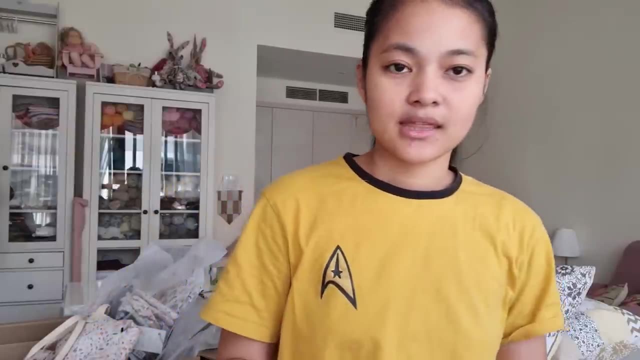 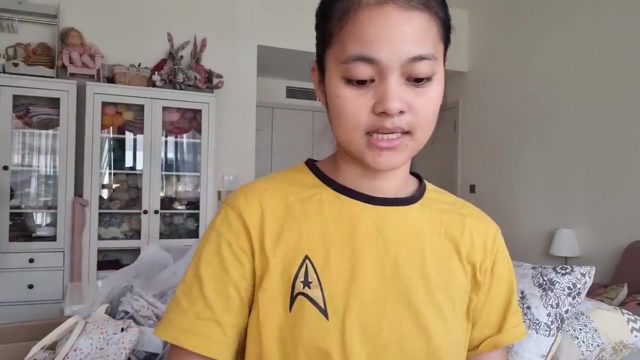 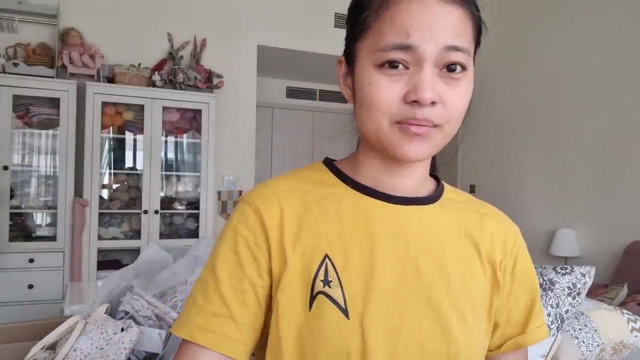 bits and bumps. it's so cool if you have an embroidery machine because you can embroider anything. and I always say that these things that are that have embroidery, especially fun words, and especially this one playing bump kit fun words- I think that's the most appealing to your customers. I mean, that's for 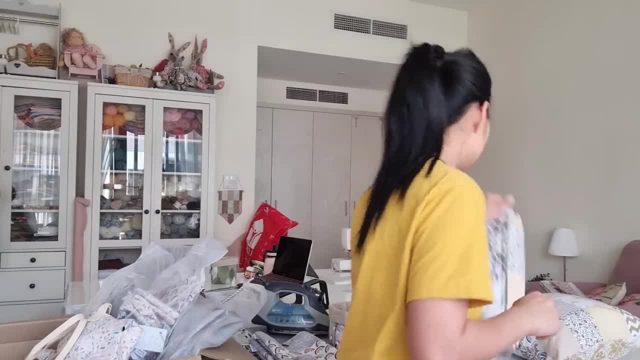 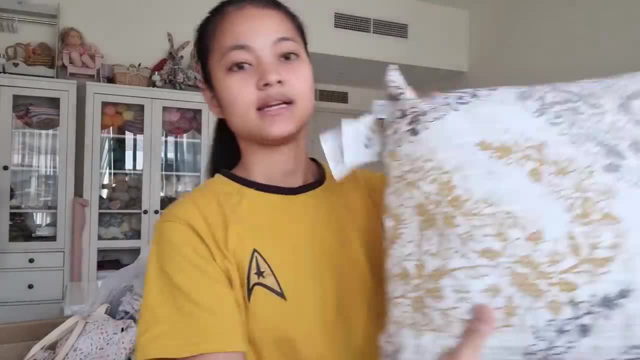 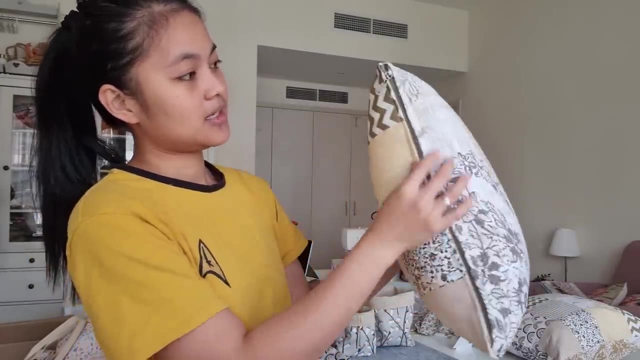 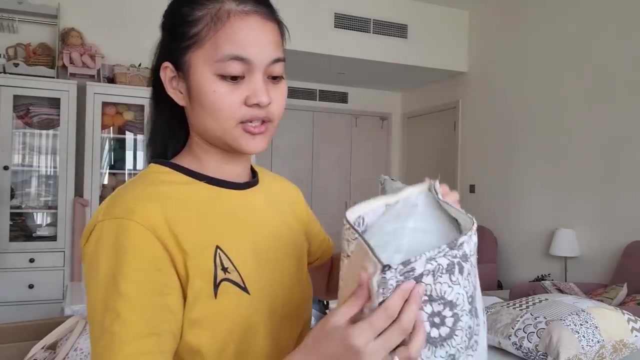 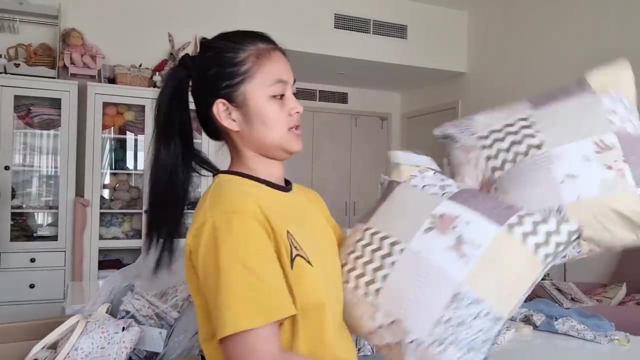 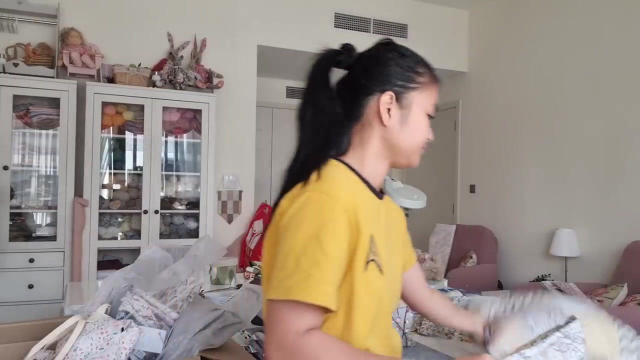 me now let's move on to. so. these are made from scraps and the back is from a curtain that my mom-in-law gave me, and it's a zip with a filler so you can wash these too, because it's- I think, it's lonely if it's only one, so I added another one. 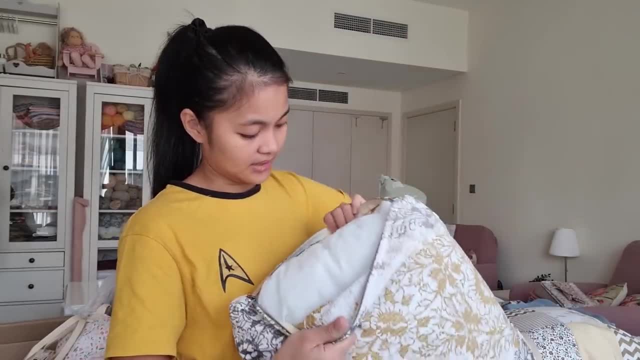 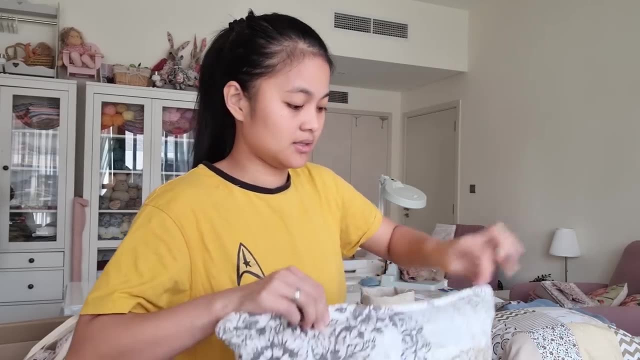 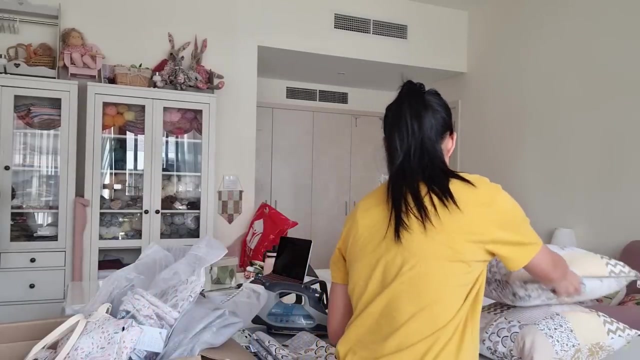 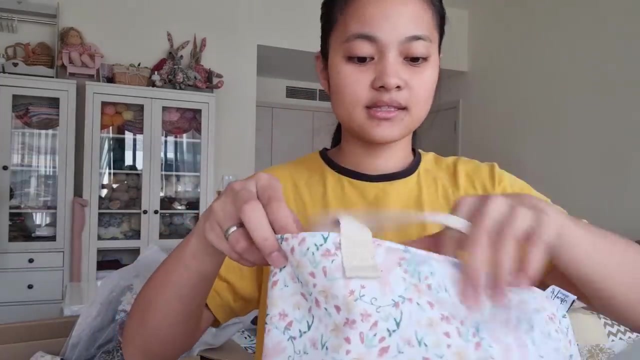 it's fully lined. it's fully lined. you don't want to see the, the stitches from the patchwork. that's not nice, it's messy. right, that's another one and I'll show you these ones. okay, I think this is the prettiest I've made for this market. well, someone. 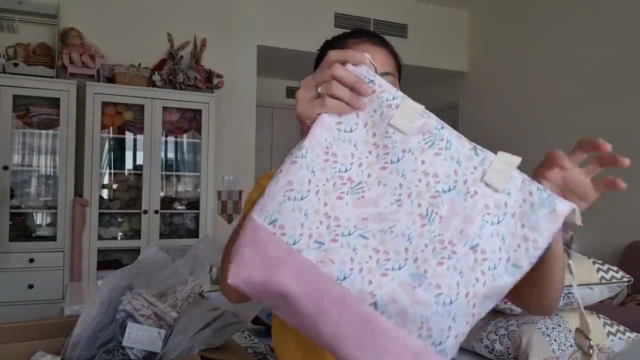 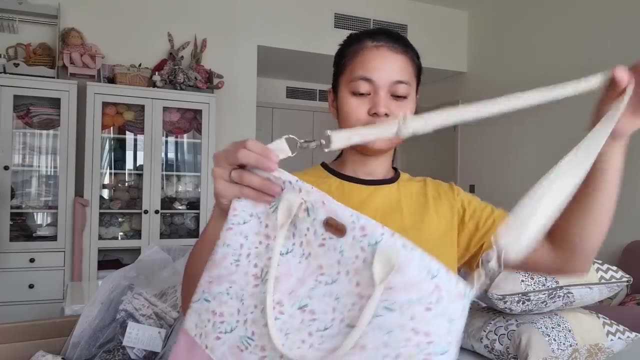 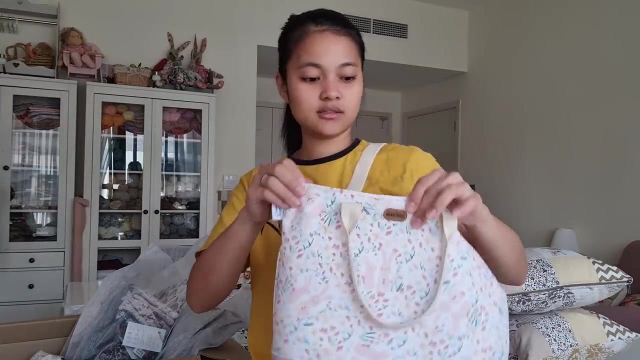 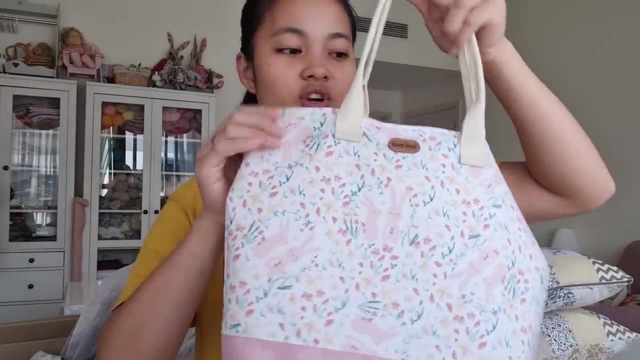 actually already ordered this and I only have one to show and sell at the market. that's okay. so I made these sling bags or crossbody or a shoulder bag, whatever you call it. these are Tote style swas квартиre discount bags. all right, of course. oh it's. 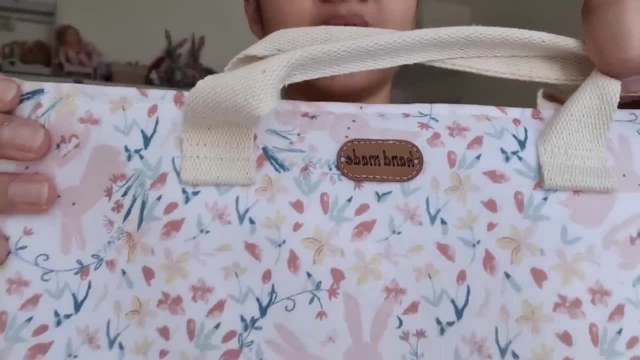 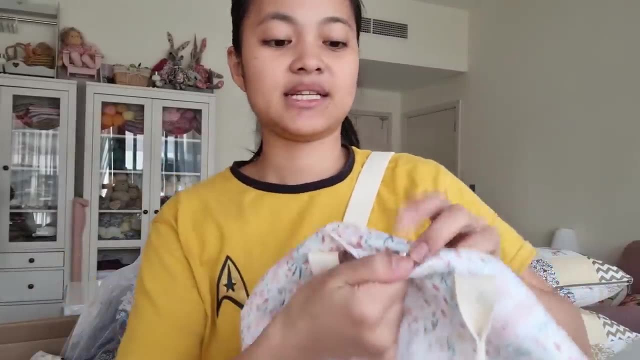 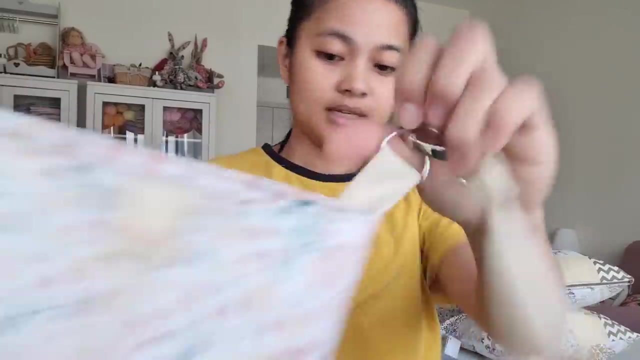 just gotten some some cool right. it's a tote-style bag and it's got this pretty handmade label. of course, all my products have my own label. yes, and this has a magnetic snap inside, has loads of pockets. yeah, also here, you can pair it with this buffalo bracelet. 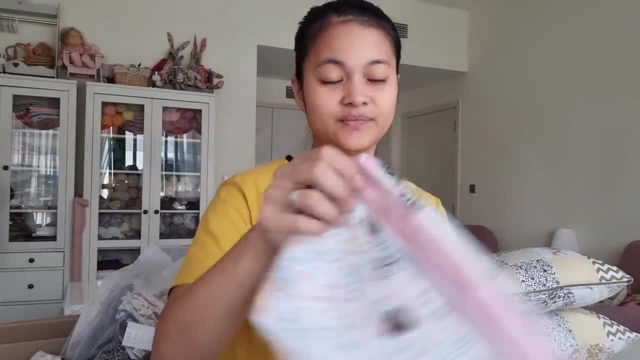 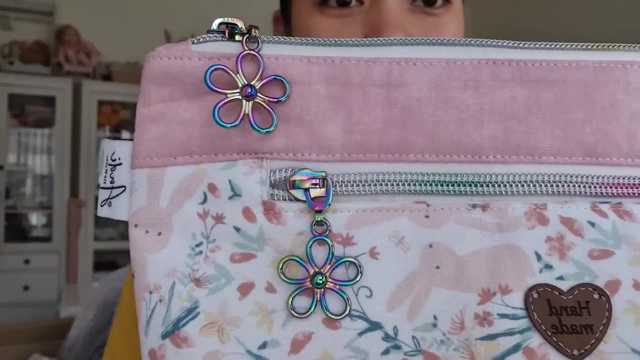 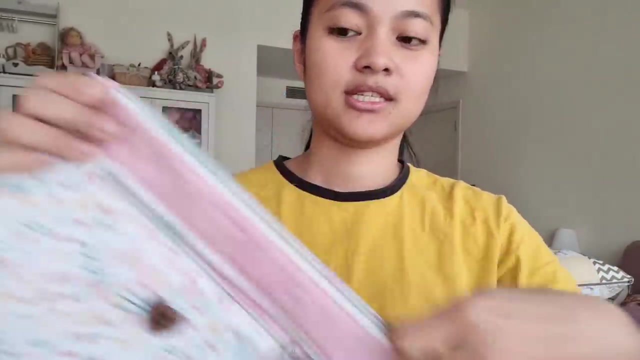 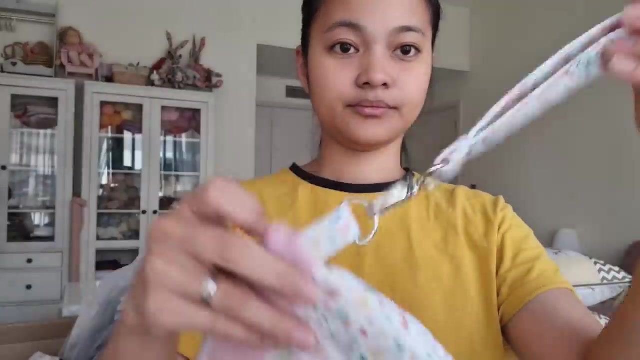 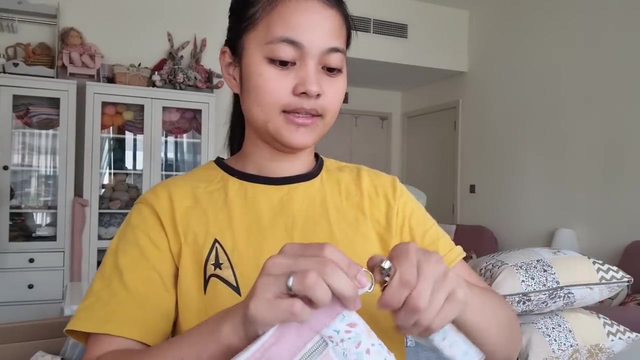 if no one buys this, i'm gonna have this. i love it. those pretty um zipper pulls and it's of course double zipped it. yeah, you can choose to not have this. you can just. yeah, easy, all right, let's move on. so that's one. i only have two sets of those. it could be. 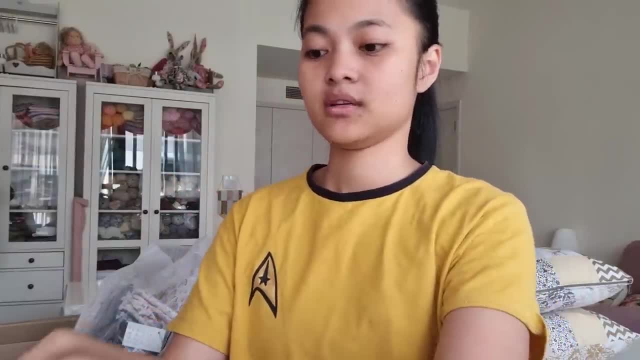 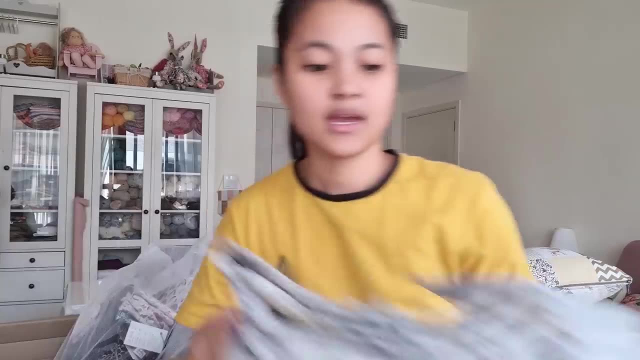 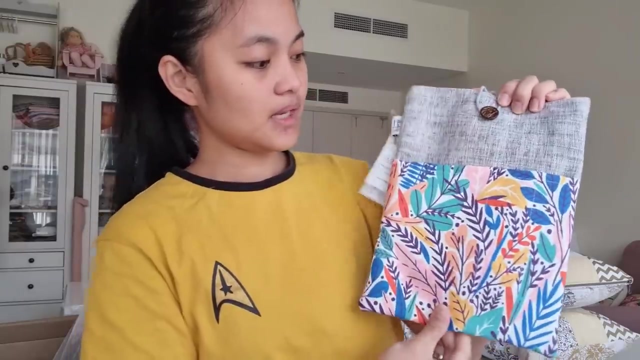 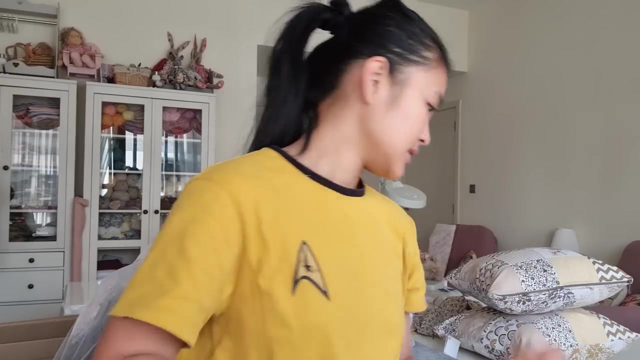 sold in a set, or it could be sold individually, whatever people like. um, all right. another thing i've made are these: it's a notebook. pouch a book. pouch an ipad. pouch whatever you call it, for me it's. you know, it's a, it's a ruler pouch. 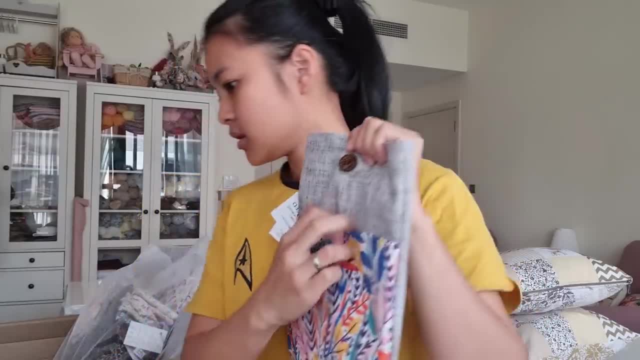 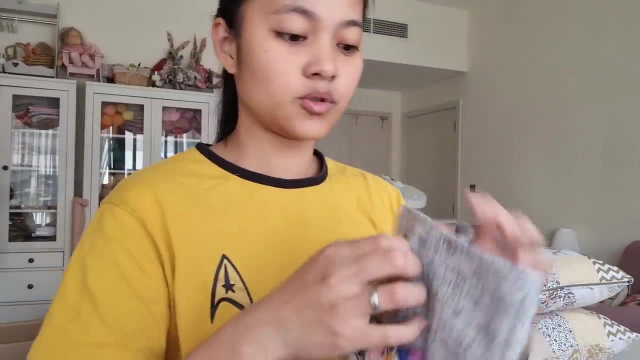 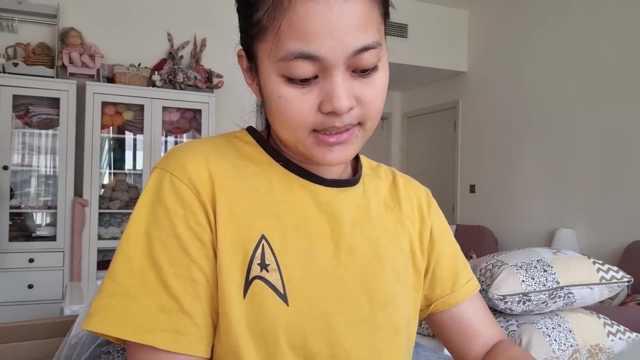 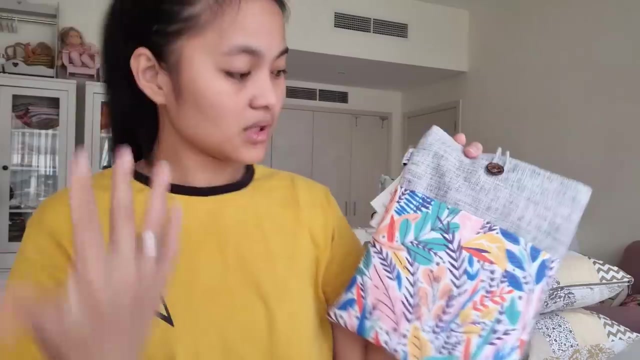 and you can put your pens in there. it's got a pocket for a pen, perfectly. and notebook, you know, very ideal for teenagers or mummies at work and likes the pretty thing. they can put it in their bag and you know it can serve as an organizer, whatever you want to do with 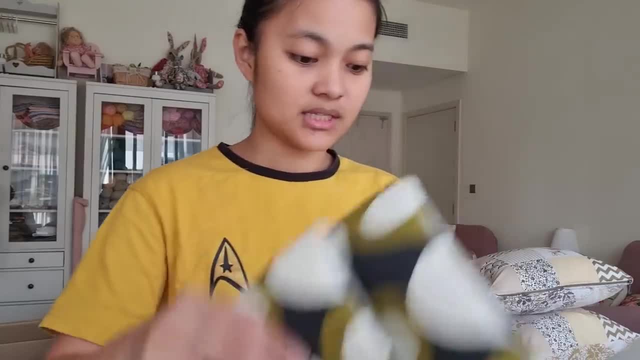 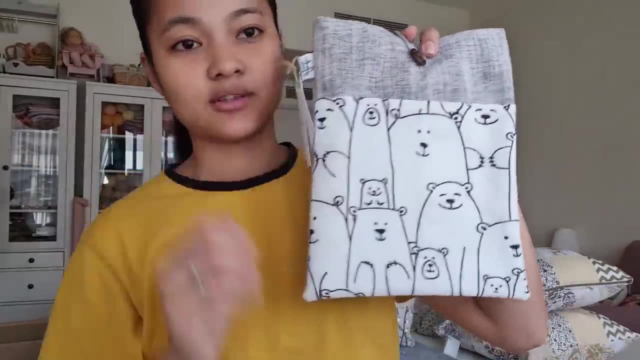 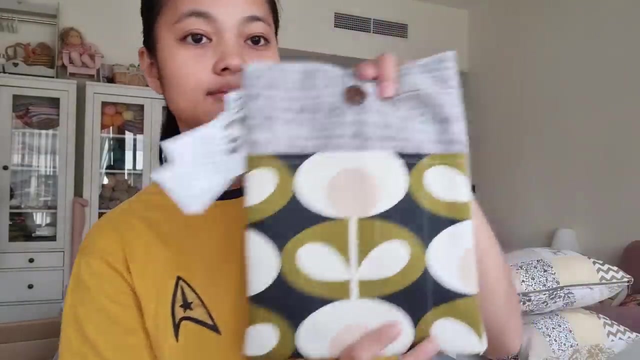 it right. i've made a ton of those in different prints. each print i made two pieces. this is another print. i think that's so cool. it's a green one and another green one. um, i've made more actually. do you want to see them? it's. 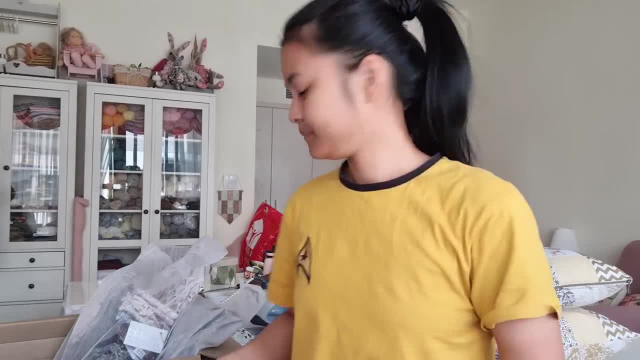 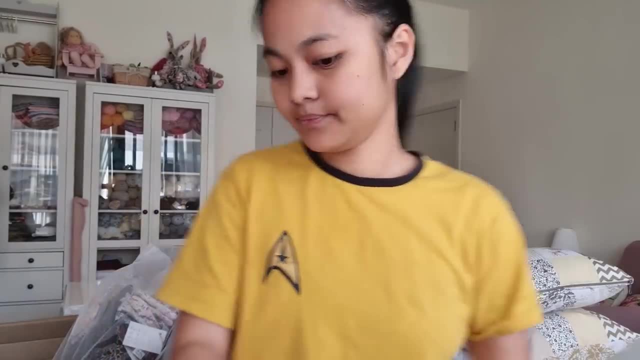 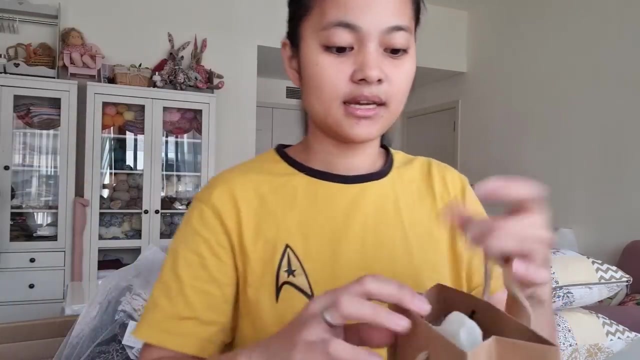 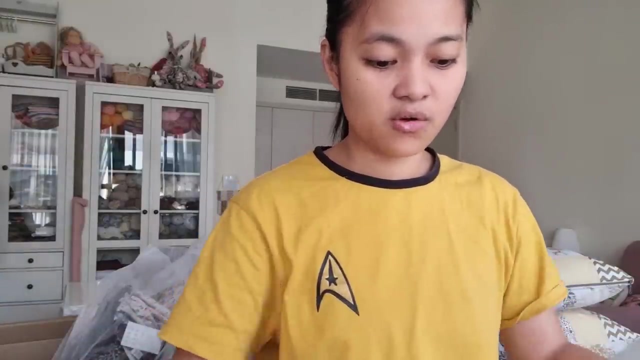 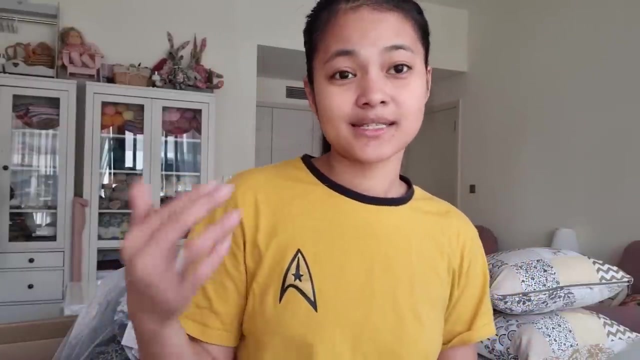 another rainbow one. i love rainbows, yeah. so that's another one. let's move on. okay, here is a- not super outside. it's something i've made before and i just thought, you know, i'll just take it with me because i made it for fun and also not just for fun- as a sample for people to see. 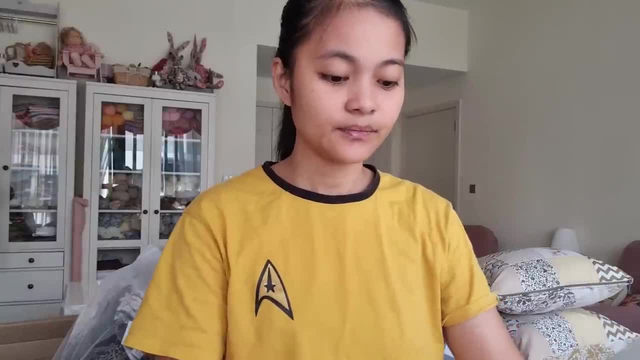 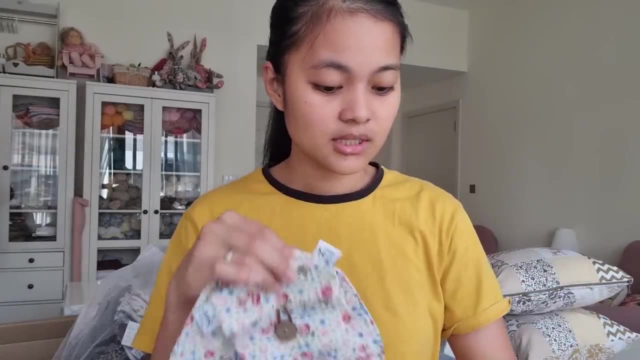 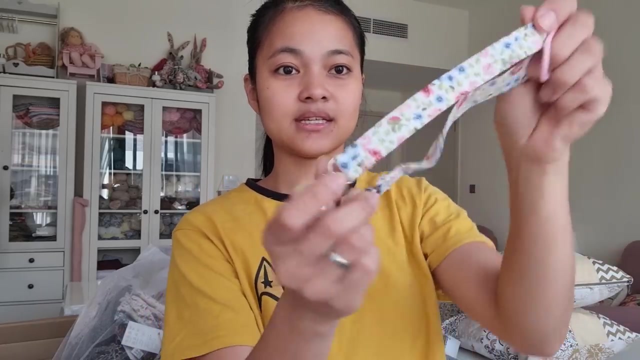 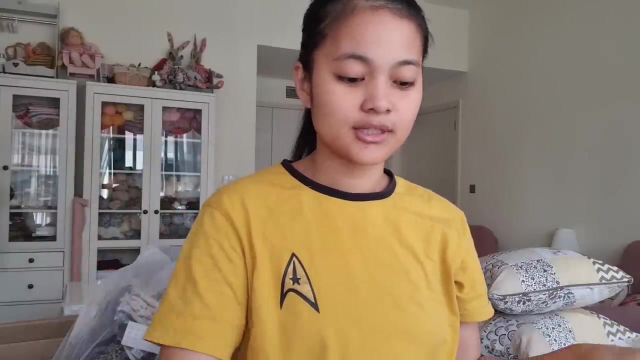 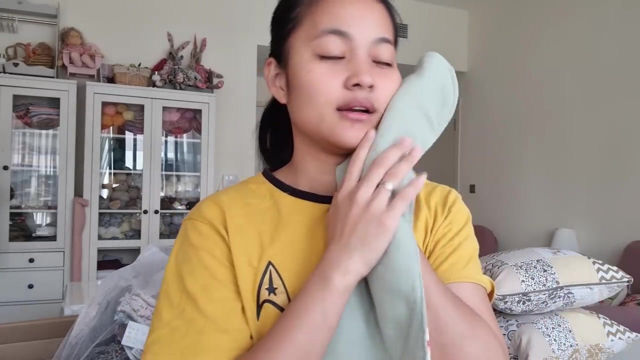 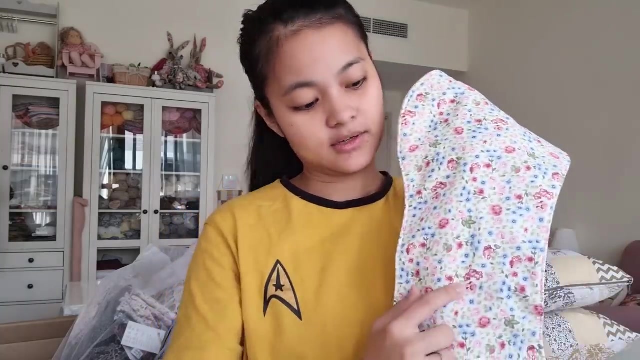 so they could order it and personalize it. this pretty bib, it's a set. this is a pacifier: pouch booty, tiny tiny booty, wow, pacifier afternoon, pacifier clips. my toddler loves his pacifier since he was four day, four day old, so we love pacifiers in. 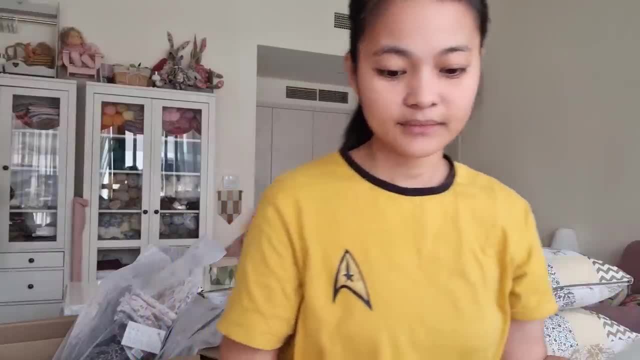 this house, um, and a bird burp cloth soft. it's double gauze on one side and cotton on another and it's got batting inside. yeah, so i'm selling that as a giftEh. patting inside. yeah, so i'm selling that as a giftEh. 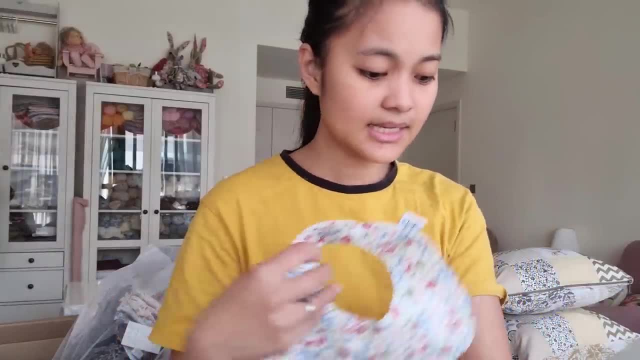 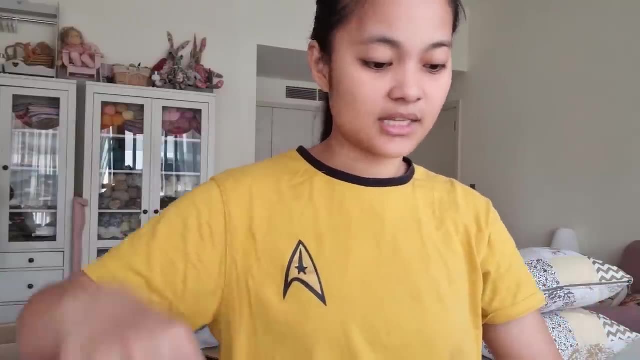 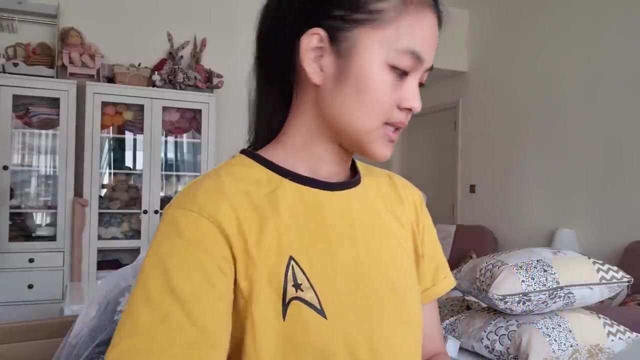 that as a set and also to show people that i make these as well and they can personalize it. they can pre-order it if they like and i'll just put it, you know, send it to their house. yeah, not everything i'll be showing at the market is for sale, because, for example, this, this memory bear, this is from my 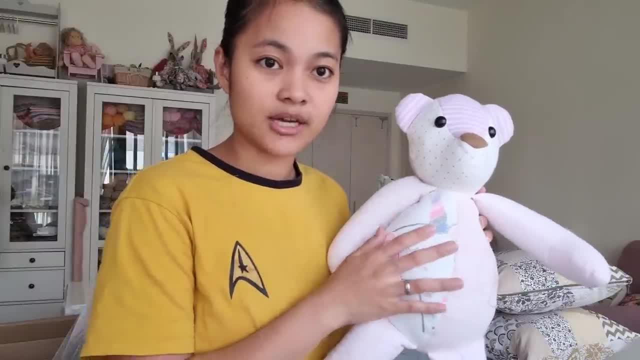 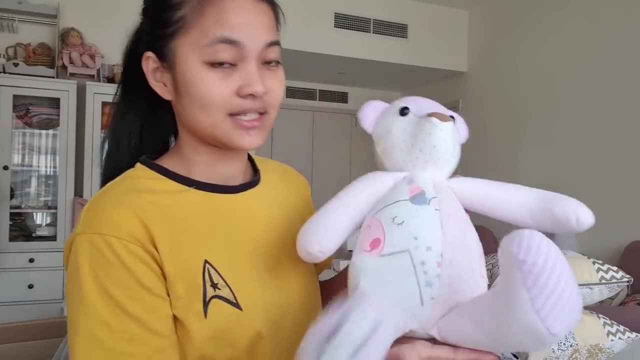 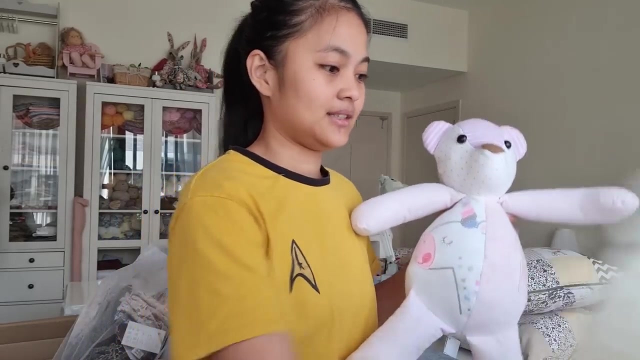 this is for a customer and i asked her permission if i could show it at the market. um, and she agreed and she thinks it's an it's nice to show at the market and she's quite proud because it's very pretty. and i agree with her: it's very pretty, um, it's made from baby clothes. 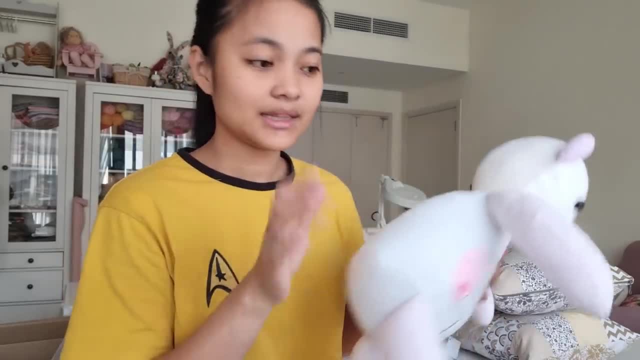 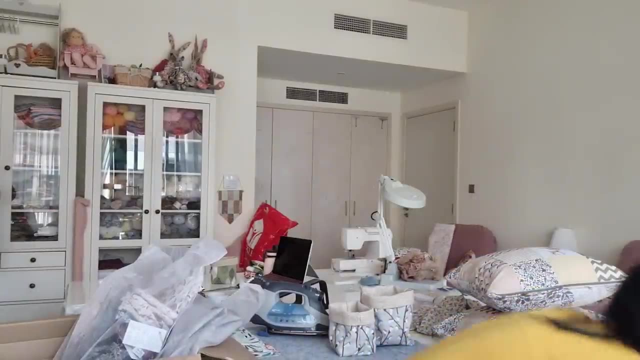 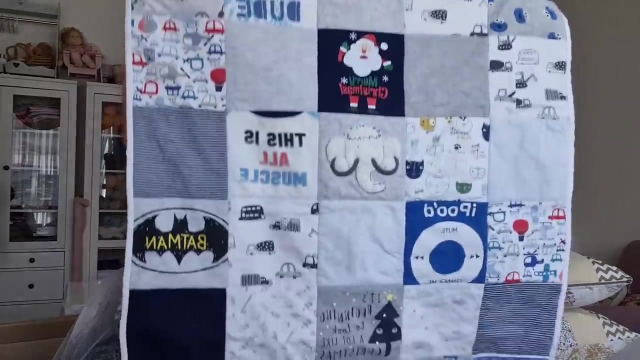 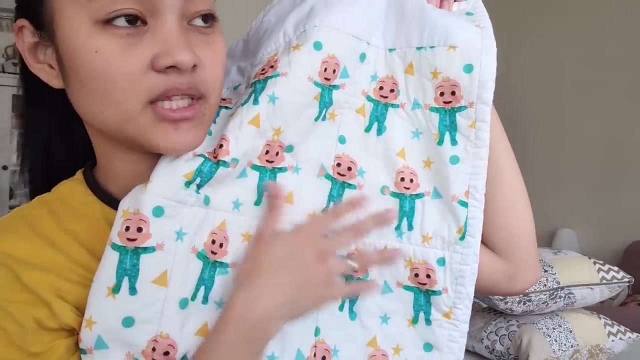 and baby blankets, yeah, so like this. i'm not gonna sell it to anyone because that's for my customer. and also, here is another one. this is my toddler's quilt. the backing is jj. if you're familiar with coco melon, he was obsessed with it for a year and then 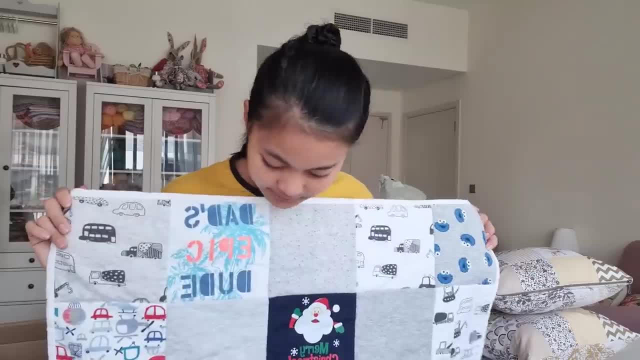 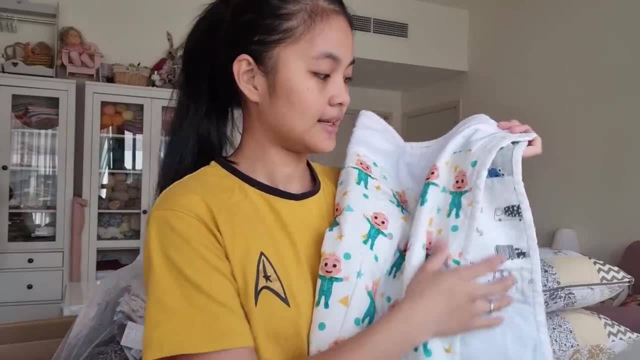 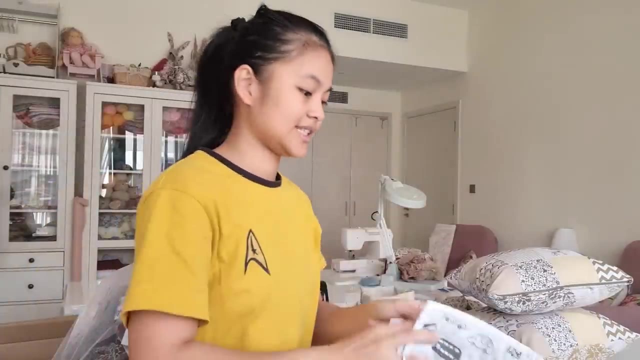 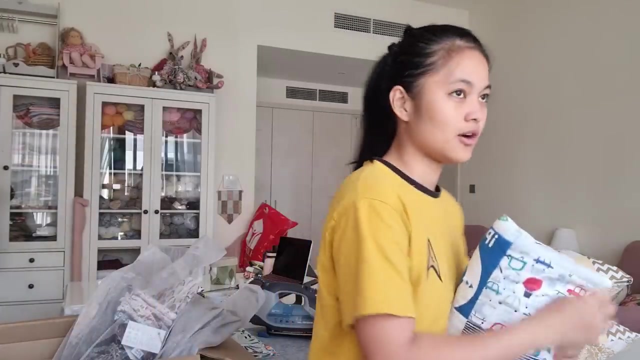 for some reason he's not that obsessed now, but yeah, um, but just a reminder that that's what he loved as a one-year-old kid, and those are all his clothes. it's a nice memory. one year, one year old, um memories, i mean the whole one year. 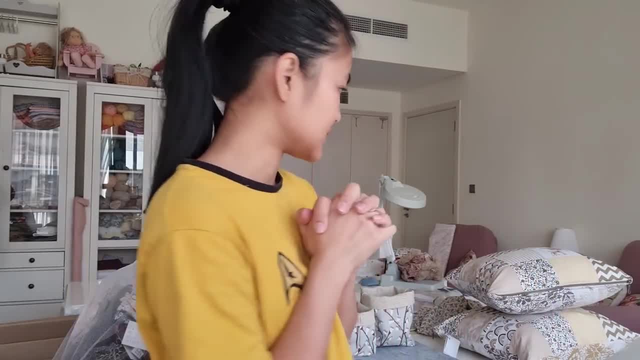 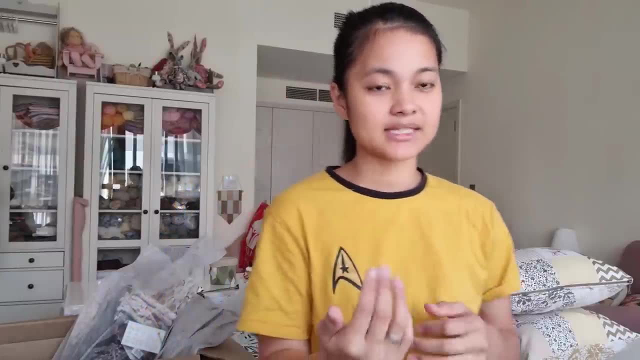 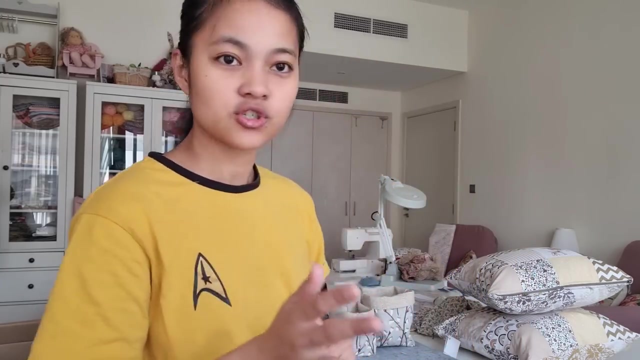 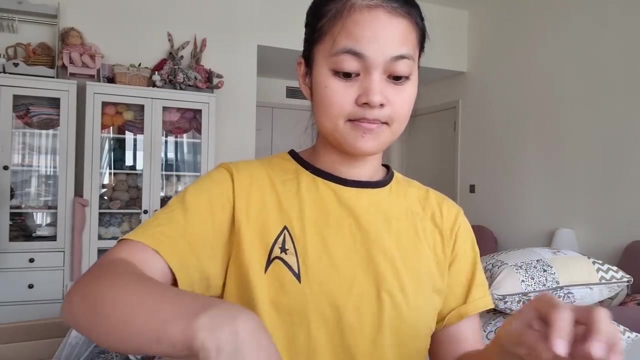 right next. what do we have next? so if you have any questions, just comment down below. and also i am planning to make a series of tutorials on all of these products. so that's coming up in the near future. near future also. this is the last item I am making today and the last one I'll be. 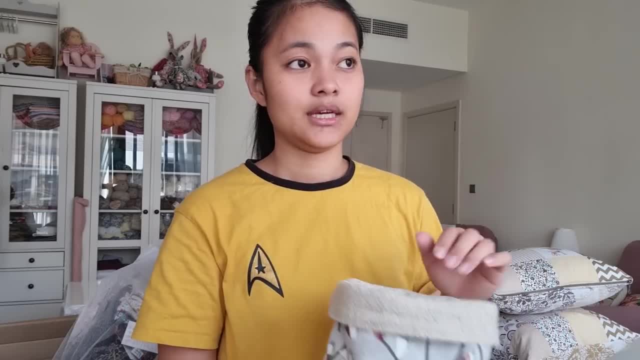 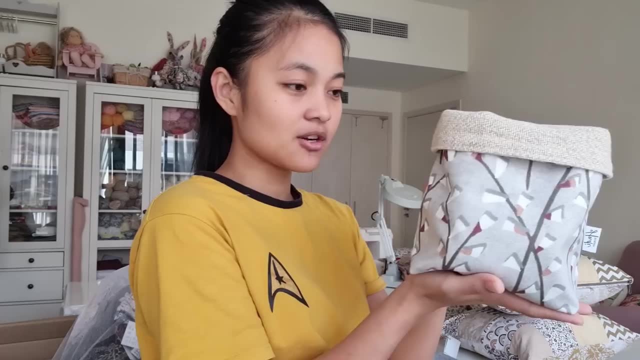 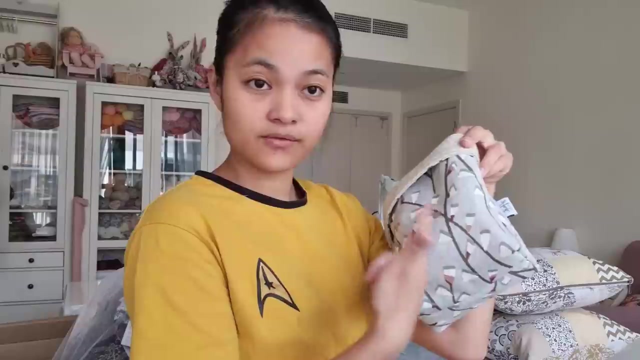 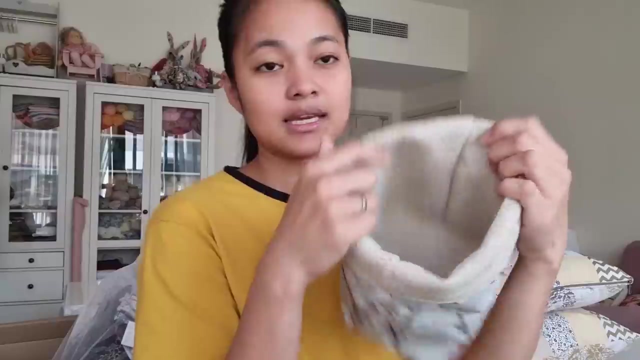 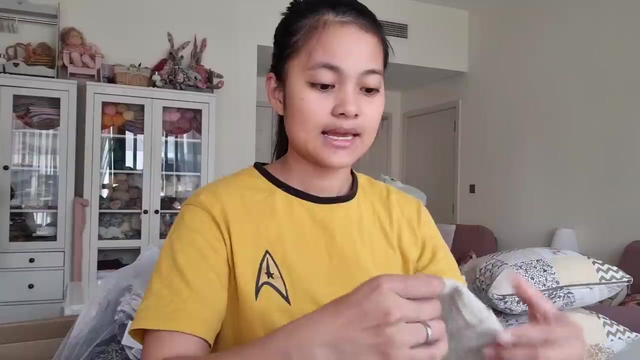 making for the market and I think I have enough. yeah, so these are fabric baskets, boxes, whatever you want to call it. it's, it's that thing. the outer panel or fabric is made from canvas fabric, but the lining is a curtain, is an old curtain that was given to me by a neighbor and it's very rough, so I 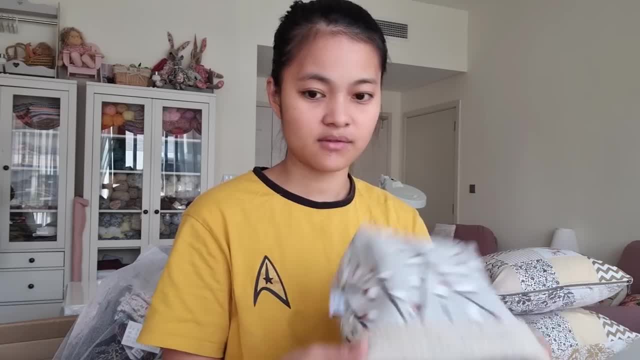 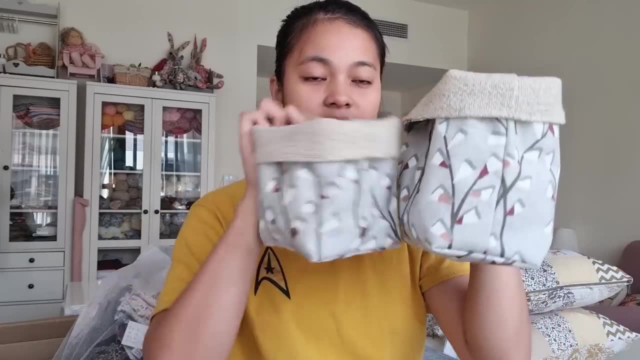 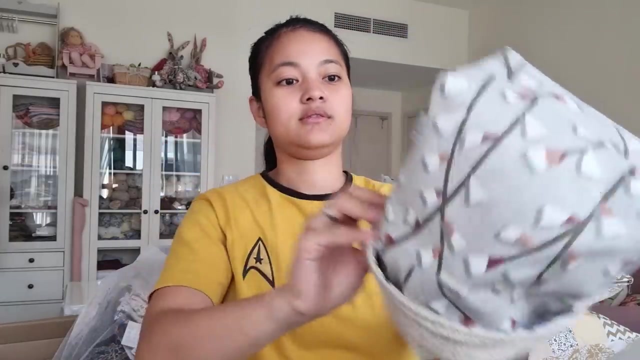 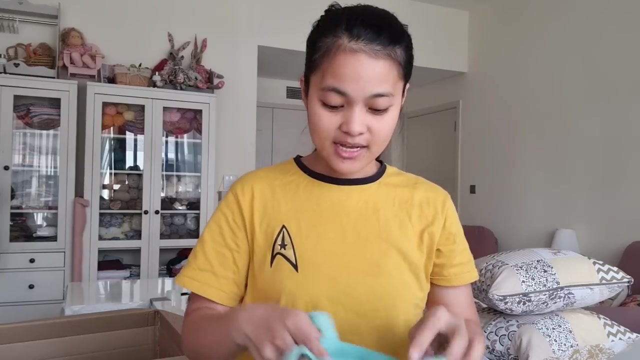 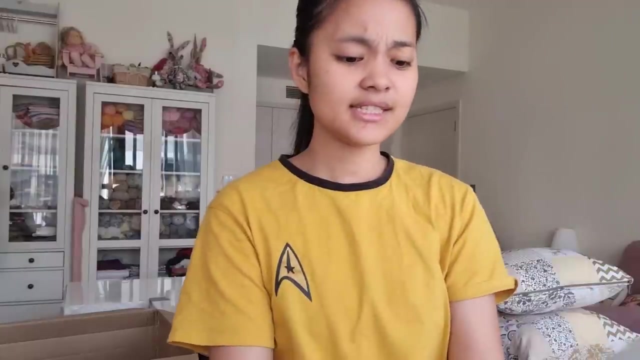 couldn't think of anything better to make out of this curtain but this fabric box. and there's a set of two, big one and a small one, and that goes easily in the big one. so, yeah, right, we had a visitor in. so next, look at these yummy scrunchies. these are not necessarily upcycled, they're. 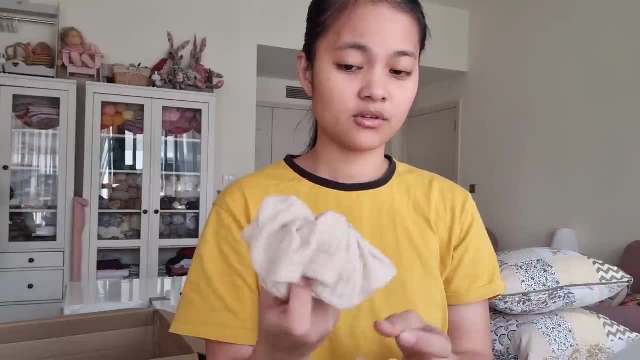 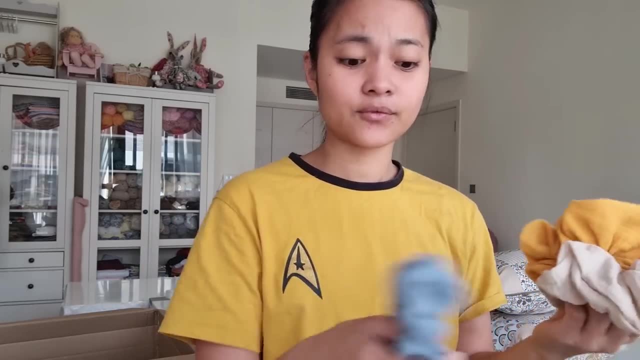 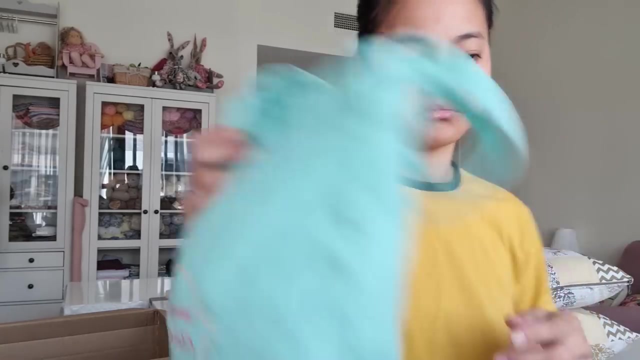 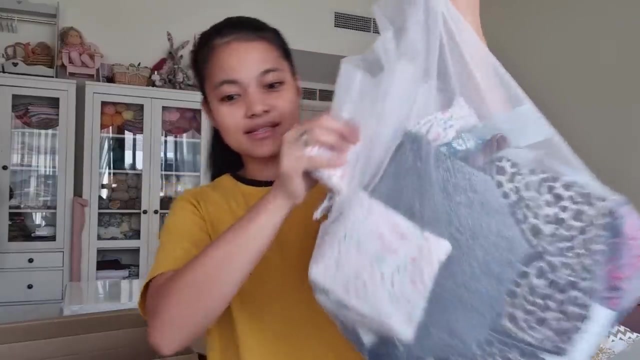 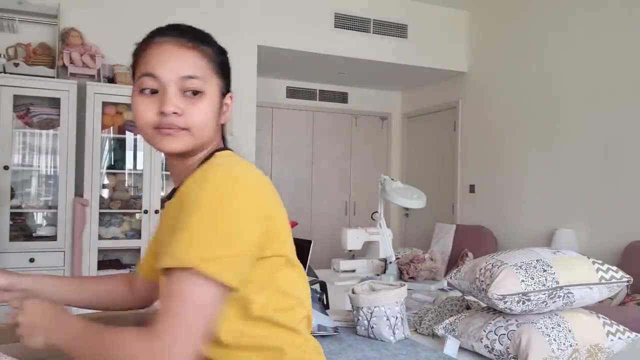 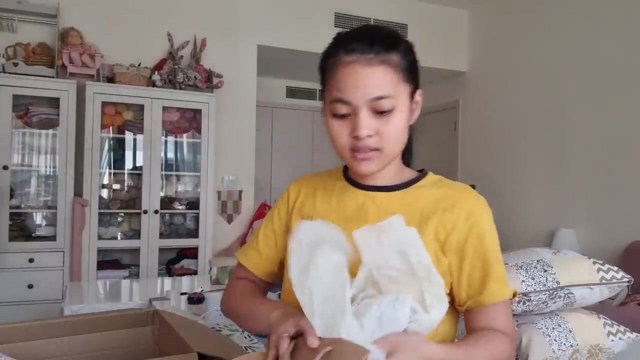 made out of scrap of muslin double gauze fabric that I had. I had them for a while and, yeah, just gonna bring them to the market and see if people like it. right next is I have a whole bag of bags. let me just tidy up a bit so I have space. I like to separate them all so easier to find. I 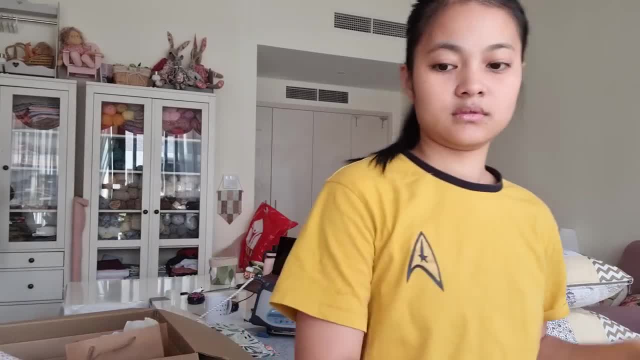 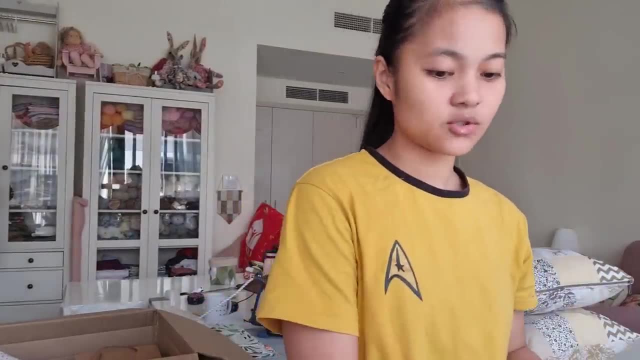 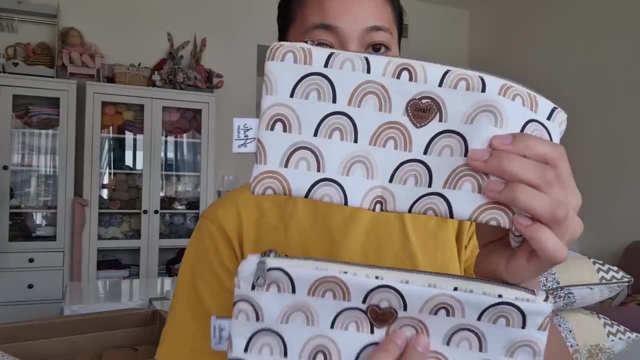 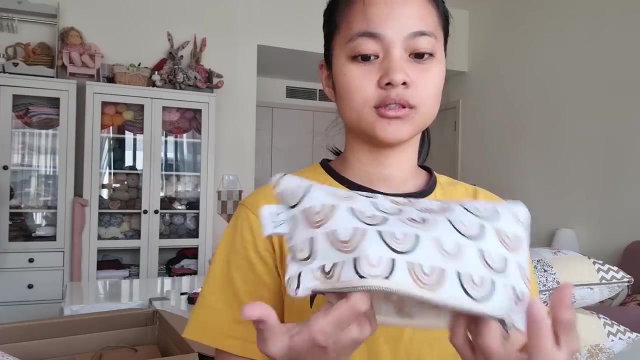 I have space. I like to separate them all so easier to find. I yeah. so now there you go. let's move on to not so upcycled ones again. these really cute rainbow pouches. they can be makeup holder, pencil holders or whatever you can fit in there. 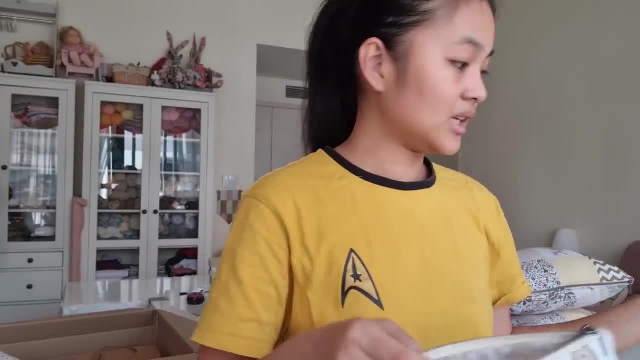 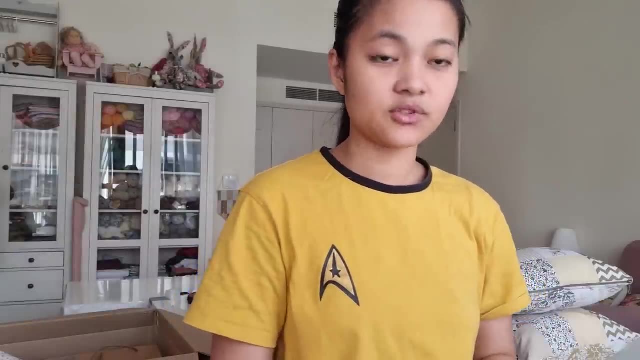 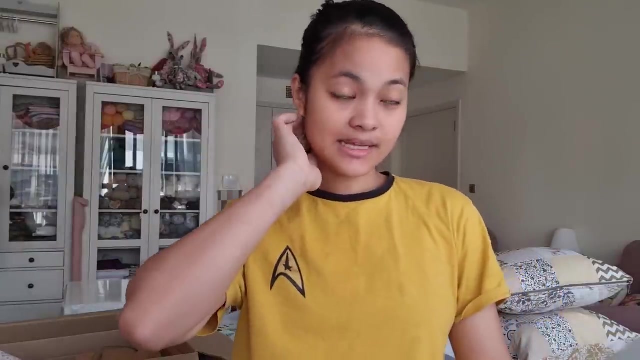 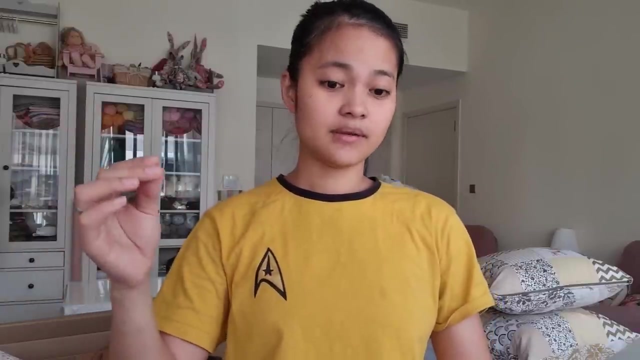 you could fit rotary cutters or anything. yeah, i have two of those. i didn't make a lot. again, i'm doing this to test the waters and if if it's successful- hopefully it will- it will be successful. i'll do it again whenever they they have their um market. 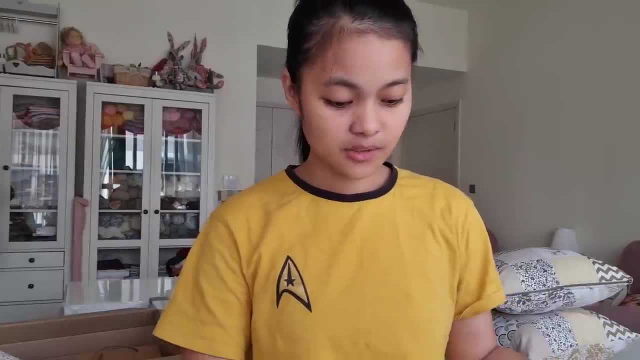 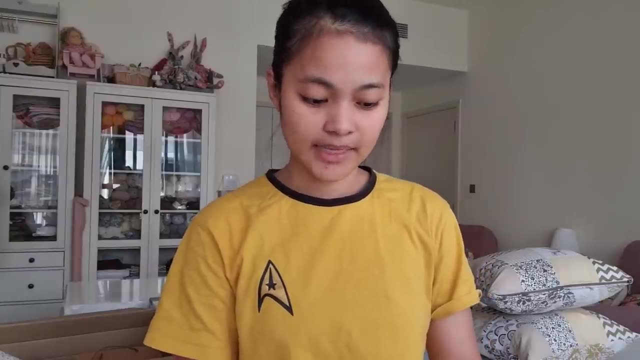 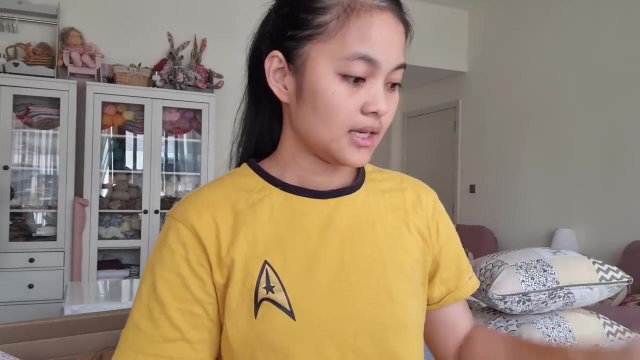 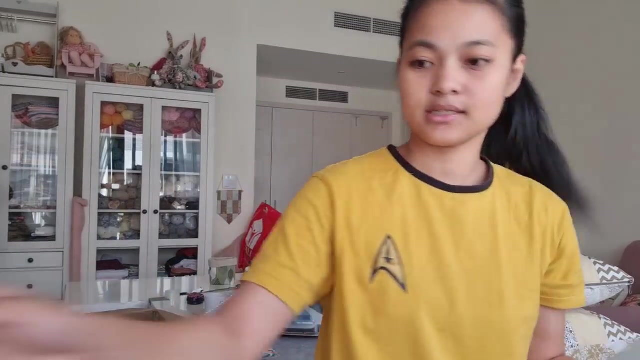 since this is the first time that the village to buy is doing an upcycled market. it's actually really nice because i'm part of it. so, yeah, that's nice, right, and i've also made these really cute ones. um, hold on, okay, that's, that's done, and also a really cute one. 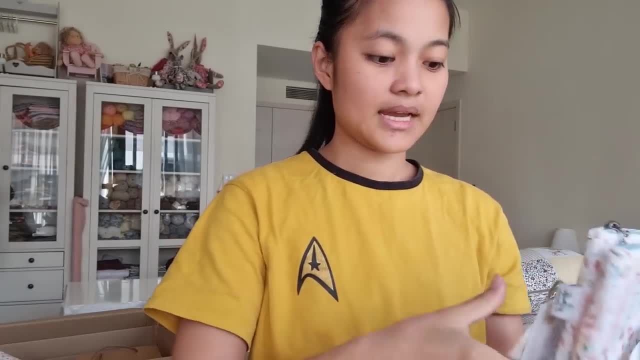 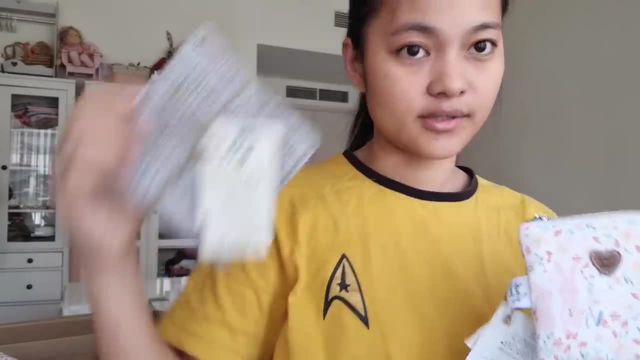 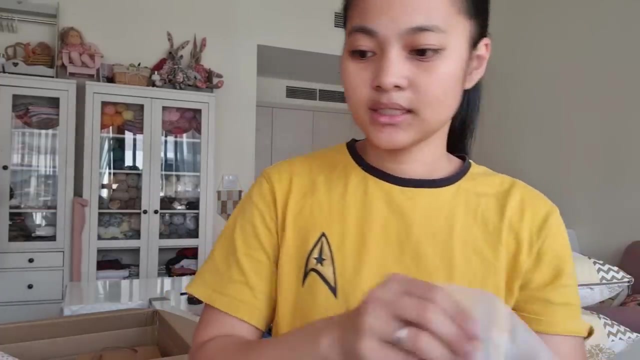 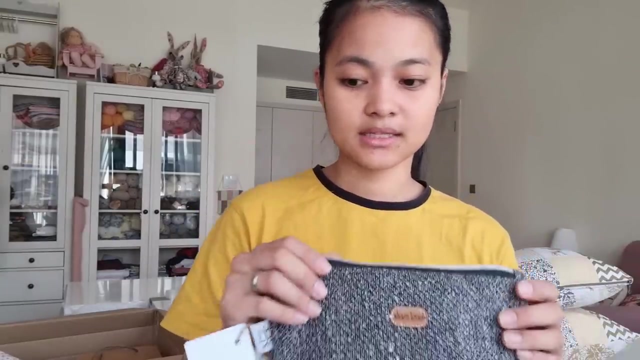 i have tags on all of them if they're not upcycled. i didn't put the upcycled tags. of course it makes sense, right, and that's just, it's just called handmade. next here now these. these ones are made from clothes, and specifically skirts. 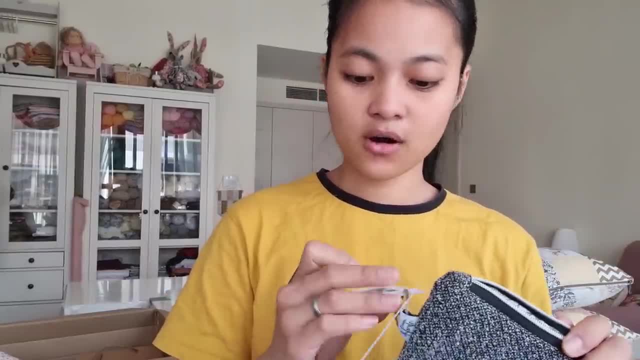 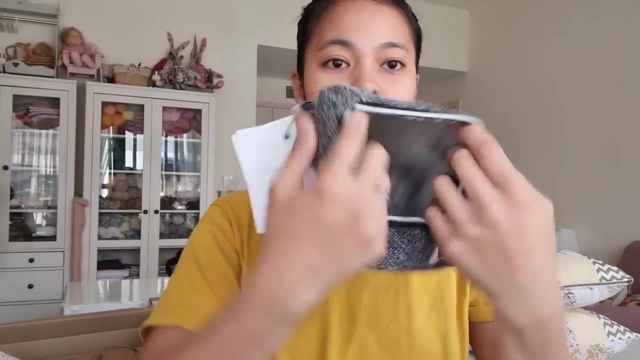 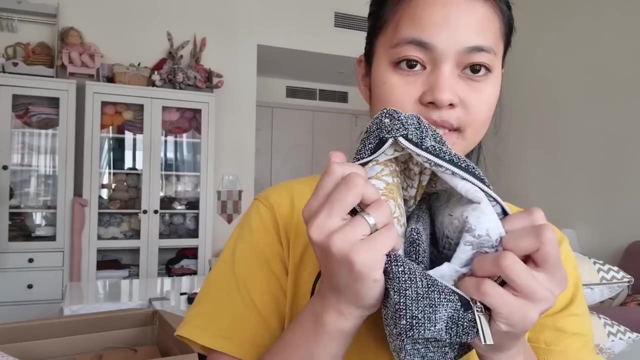 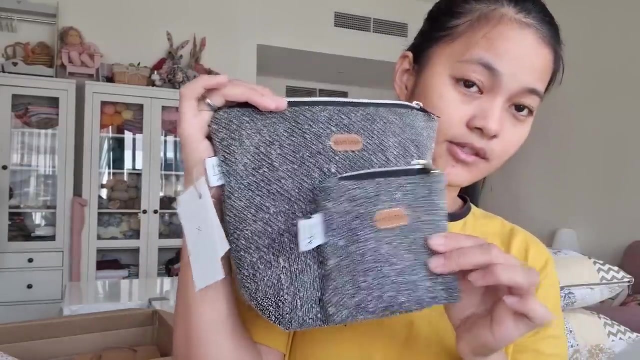 so for people to know and to see where they're from. i've actually printed a photo of this skirt and the lining of all these pouches coming coming up are from a curtain. so it comes in two sets, a tiny one and a mama one, so it could be a mommy and me ones, or? 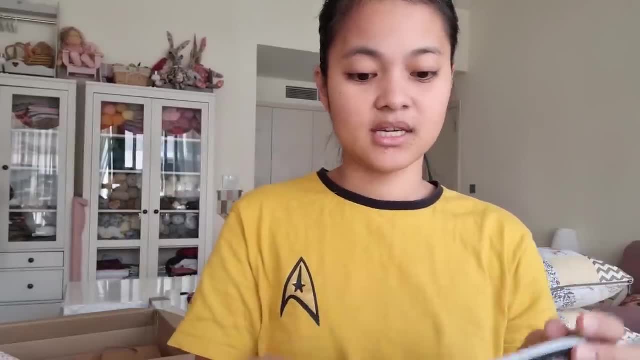 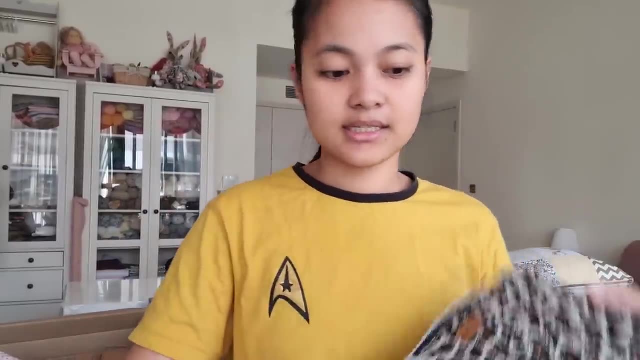 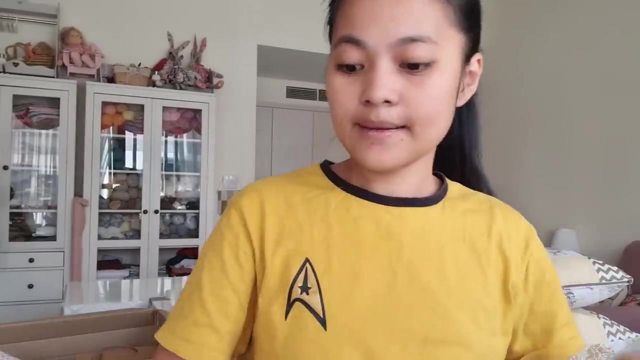 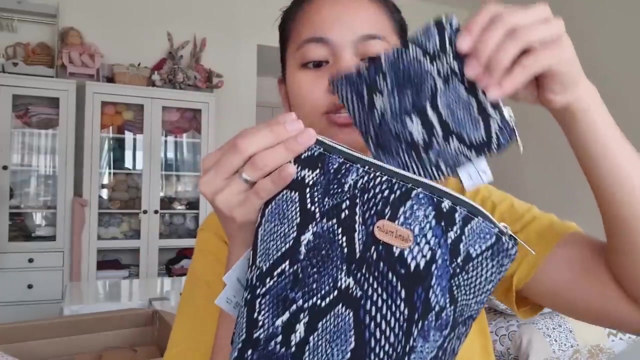 you could just have it both for yourself, whatever you want to do with it, and you can put it in your big bag or just have this as it is next. this, this nice print, and another one, um, oh, this one, another one. i tried to make sure that i'll. 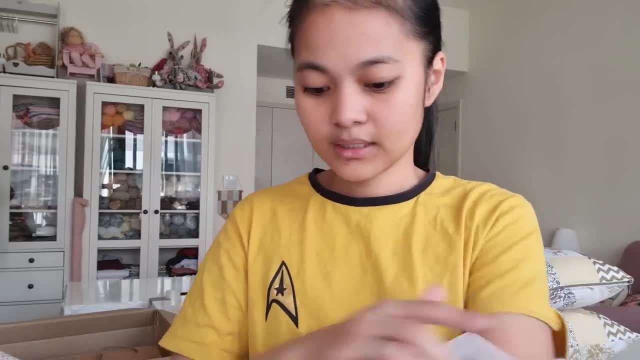 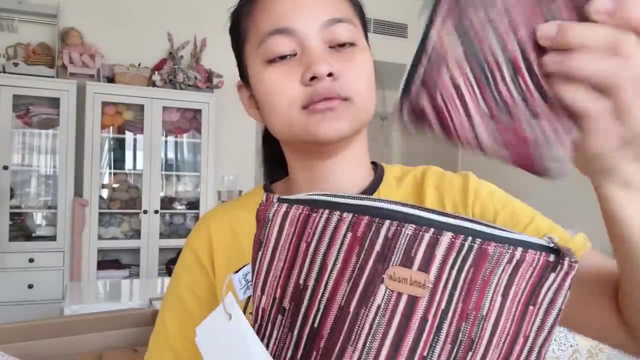 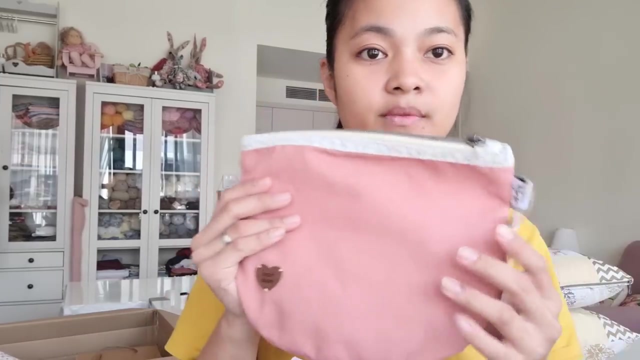 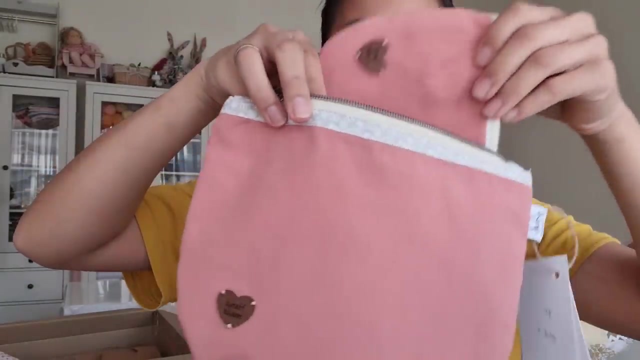 i have a set of two and a lot of people like this one. yeah, i quite like this one, and this is made from my blouse, so this is very personal to me. it's a different shape, it's a small one and a scrunchie who doesn't like a set. 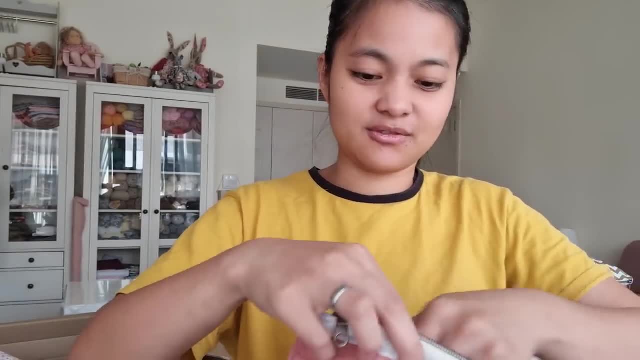 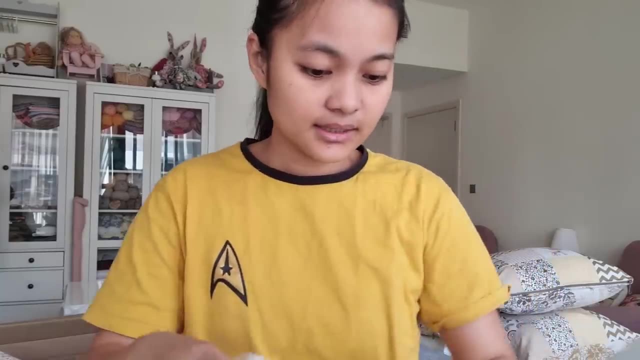 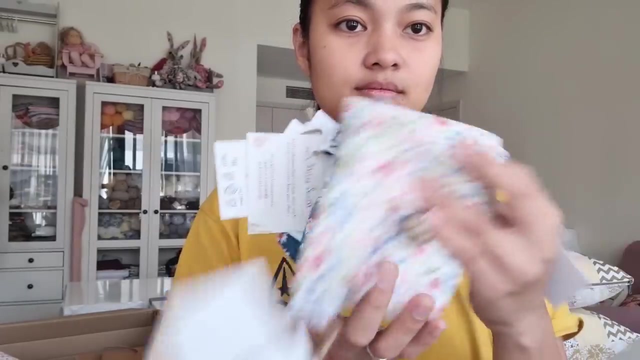 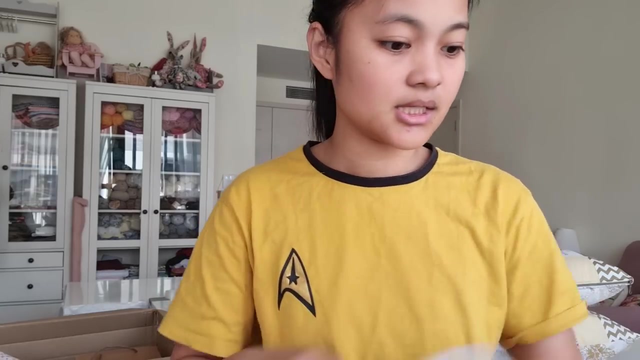 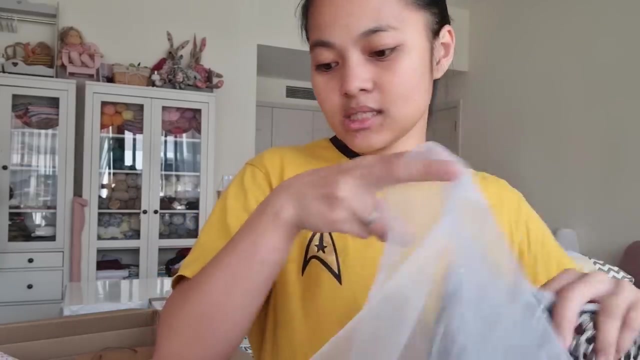 a matchy matchy ones. everybody likes a matchy matchy ones, right, and yeah, these ones are again. you saw it earlier, just a tiny pouch. i've made these before, so not last two weeks, but from my previous markets, and those are the leftover ones. just gonna take it to with me, so let's see people like it. 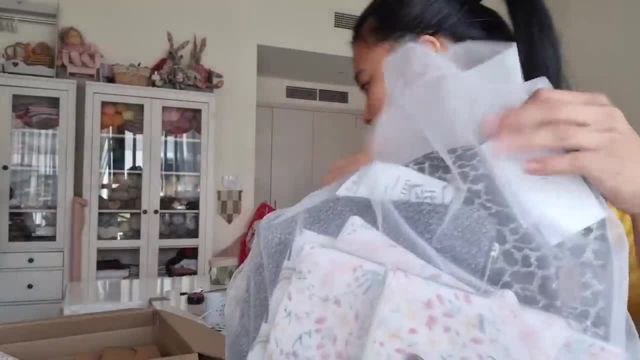 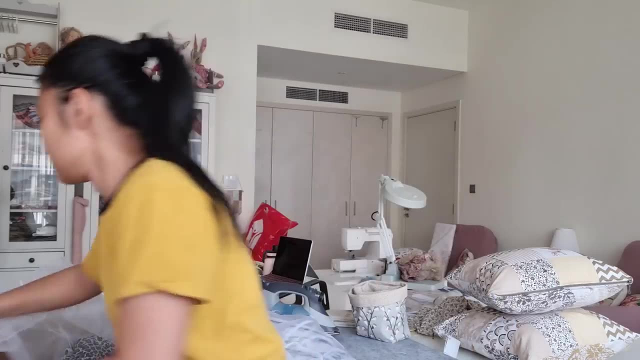 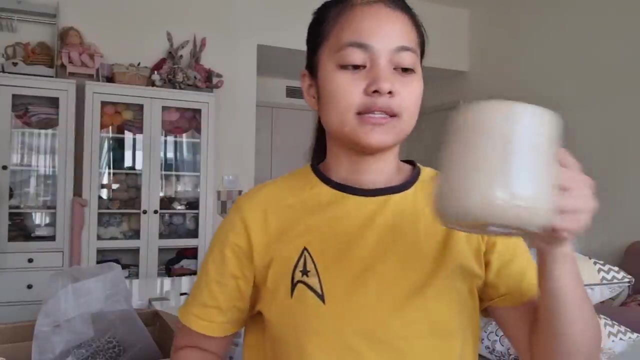 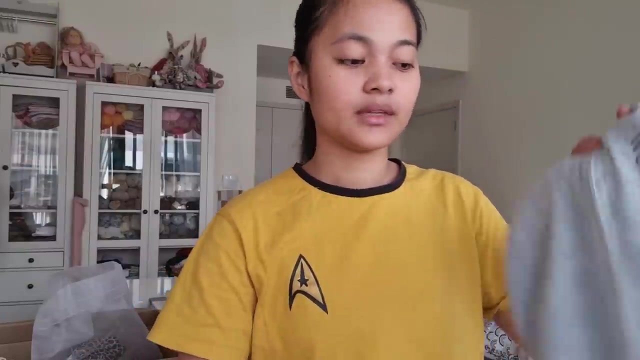 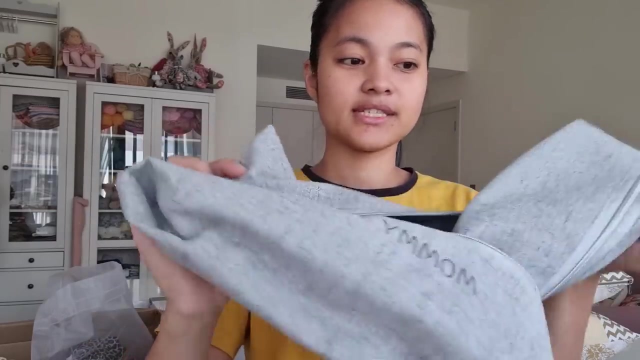 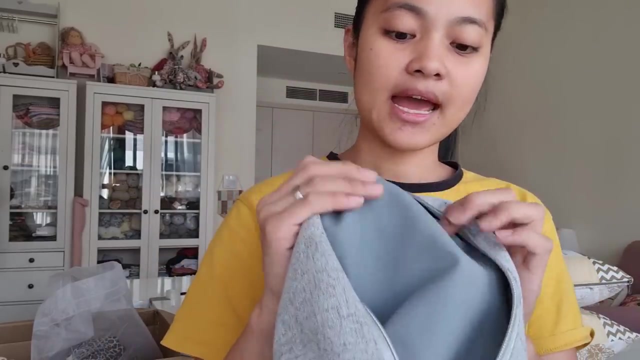 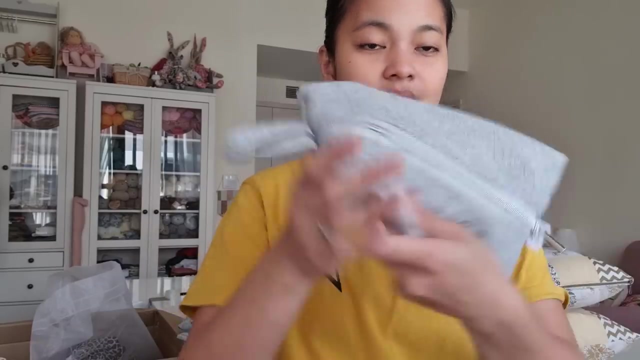 yeah, so i like to put them in this bag, just to separate them all. okay, last ones, i think last ones. yeah, these are the last ones. okay, let's take a sip right. next one: mommy things and- and you guess you're right- baby things. so this again has a waterproof feel and it's from a curtain.